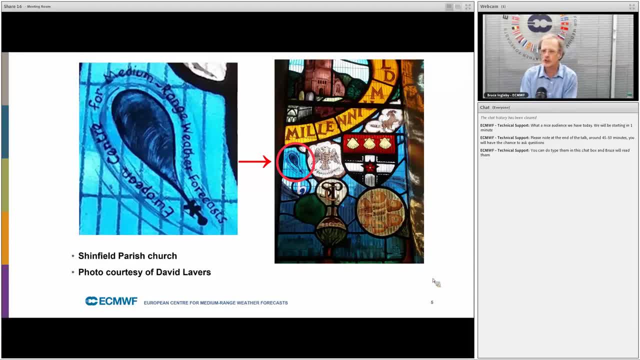 to discover at our local parish church they have a millennium window including an image of a radius on and as a sort of indication of what's going on in the UK. So I'm going to give a little bit of an introduction of ECMWF's presence in the parish. Anyway, on, 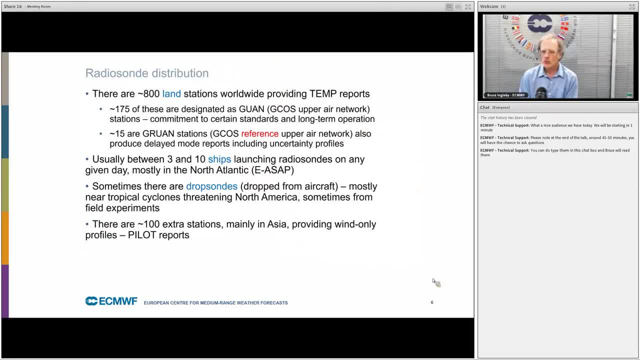 with the main talk. There are about 800 land stations worldwide. 175 are designated as Gouan or climate upper air stations, and 15 are Grouan or reference stations. There are a number of ships that are in the Parish. One of them is the Gouan, which is a ship. 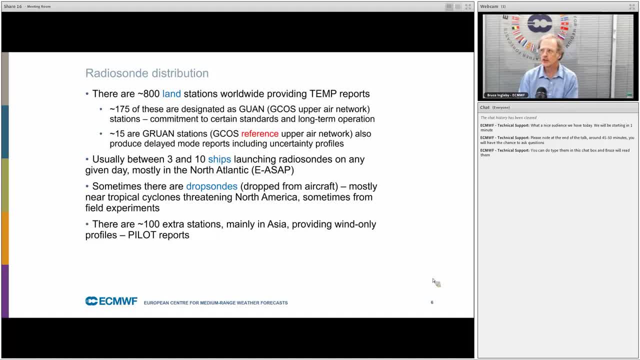 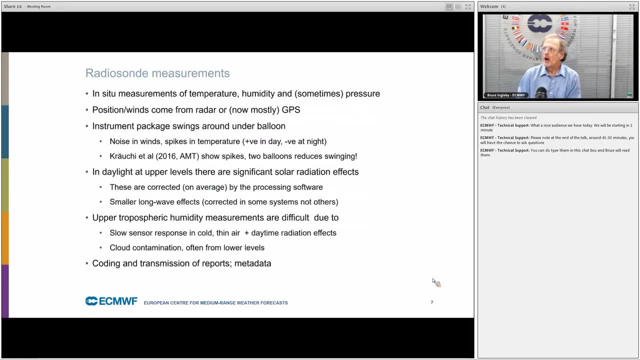 that features the teachings of Gouan, and the Gouan is a ship that's been indicated as the best place to pick up, so the Gouan is a very traditional destination as far as Pointe-de-France goes. I'll show you a picture of one of the ships that has been listed as the best place to pick. up on the Memoirs for March 21st. The first ship I believe is on the East Coast of England- It's a Gouan, So it's in Northern Ireland and on the north of the country It's through the sea around the. coastline and is seen between the river and the sea. That's a Gouan. The first ship is a light ship, though it's a Gouan. The last ship is a Pacific. Kestrel-ий-YAF was first sent in August and it's a Gouan ship. 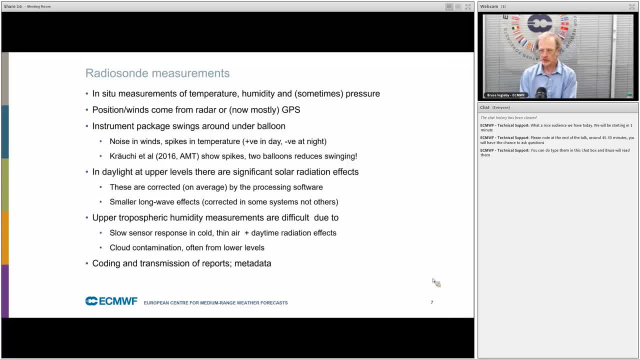 and some have a pressure sensor and others don't. Position and winds used to come from radar. now in many cases it comes from GPS. There is an instrument package which swings around under the balloon and this swinging does have effects. You get noise in the winds and spikes in the temperature. 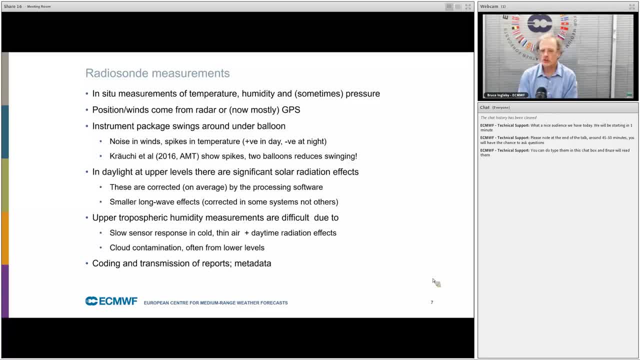 which the spikes tend to be removed by processing In daylight. at upper levels there are significant solar radiation effects- I'll say a bit more about those- And upper tropospheric humidity measurements are difficult because the sensor reacts more slowly in very cold conditions. and there are also 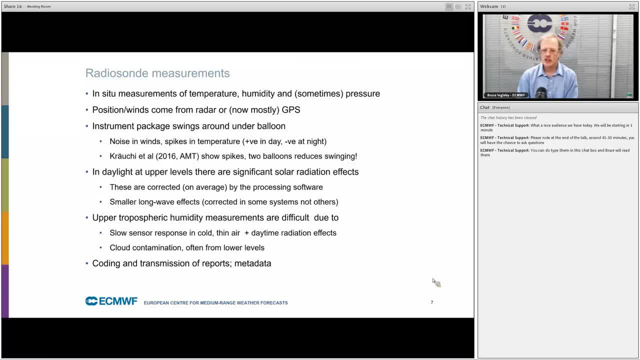 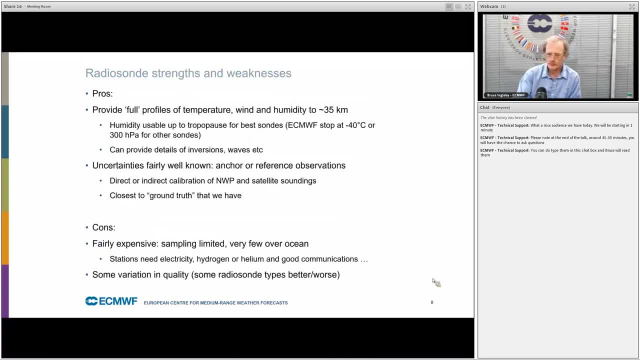 radiation effects and, in some cases, cloud contamination from icing at lower levels. Something about the strengths and weaknesses of radiosondes. they provide full profiles of temperature, wind and humidity. The humidity is more difficult at upper levels. as I've said, For the best radiosondes it's 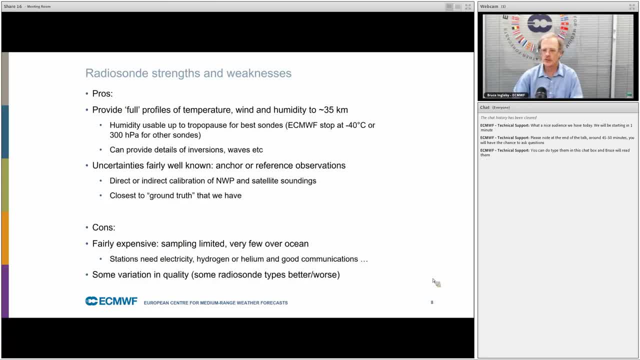 usable up to the tropopause. For others, ECMWF uses it until a temperature of minus 40 Celsius or 300 hectopascals, And radiosondes can provide a lot of detail in the vertical. I'll show an example: The uncertainties of radiosondes. 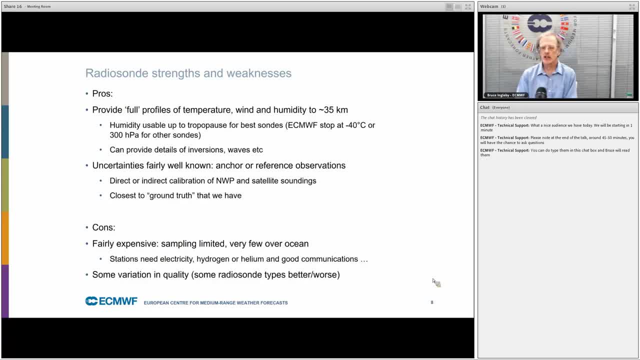 are fairly well characterised and they act to anchor. the NWP system can be used for climate reference and indirect calibration of satellite soundings And in general they're the closest to ground truth that we have. They are fairly expensive, which limits the sampling. 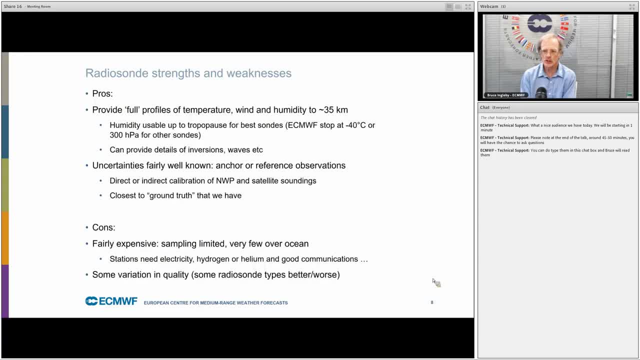 We get rather few over the ocean and you do need access to electricity, gas and good communications, and at remote stations these can be a problem And there is some variation in quality. Some radiosonde types are better than others, So this is an example of the. 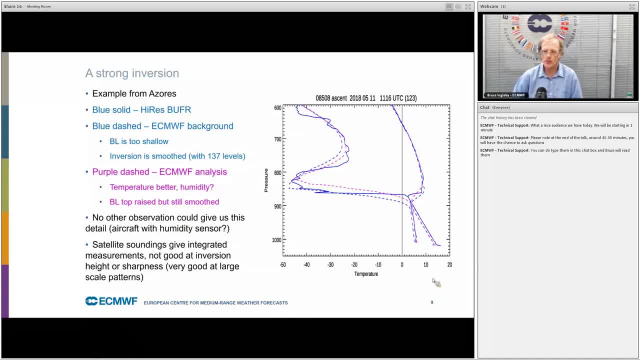 kind of vertical resolution that a radiosonde can give. The solid blue line shows a high resolution radiosonde ascent with a very strong inversion. This is temperature and the dewpoint temperature. The blue dashed line is the ECMWF background or short range forecast. 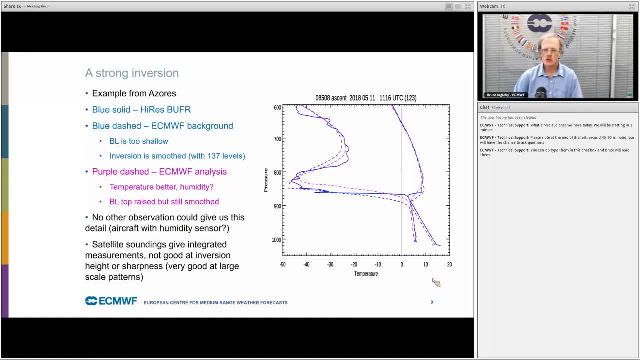 And you can see two things here: That the boundary layer is too shallow in the forecast and it isn't as sharp as in the observation. The ECMWF model has 137 levels, which is state of the art, But it's not sufficient to capture. 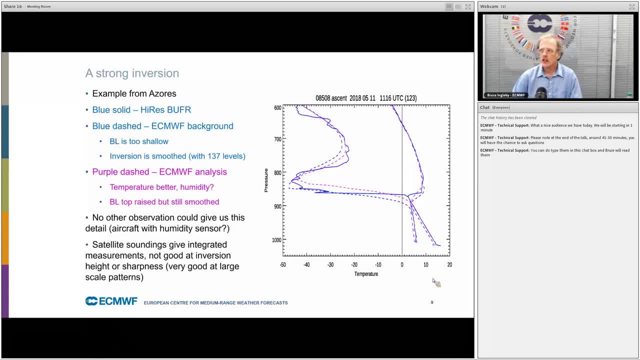 the sharpness of this feature, The analysis, the purple dashed line gets the boundary layer depth a bit better and it certainly improves the temperature. You can argue about the humidity, And no or very few other observations could give us this level of detail, for example, 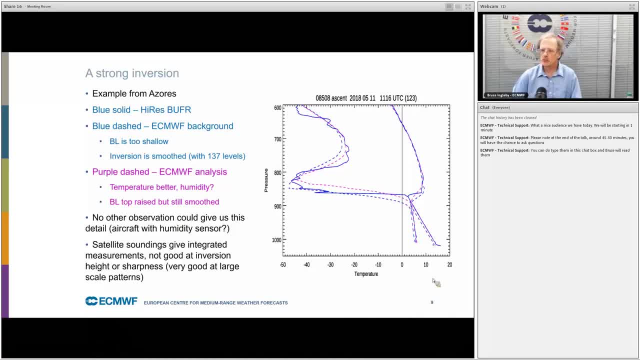 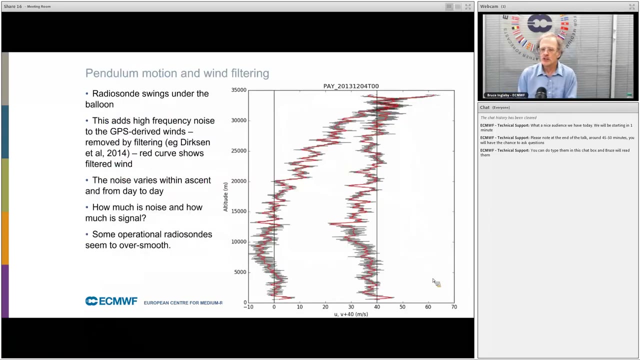 satellite soundings give integrated measurements which are not good at telling you about inversion, height or sharpness, And in an assimilation they will tend to move the temperature profile left or right rather than move the top of the boundary layer. And I mentioned the pendulum. 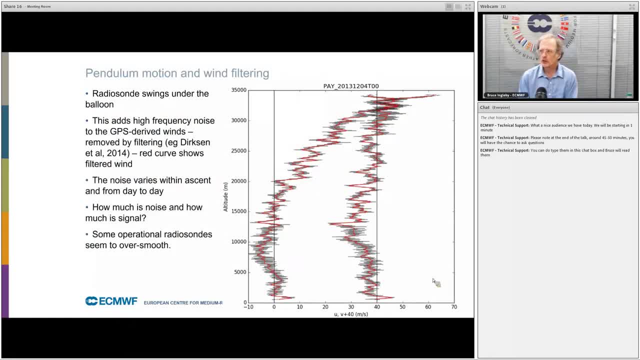 motion. This shows the U and V wind components offset The light. the grey curve shows the instantaneous winds and the red shows the time average winds which are intended to, and largely do, take out the high frequency noise, as you can see to some extent from this. 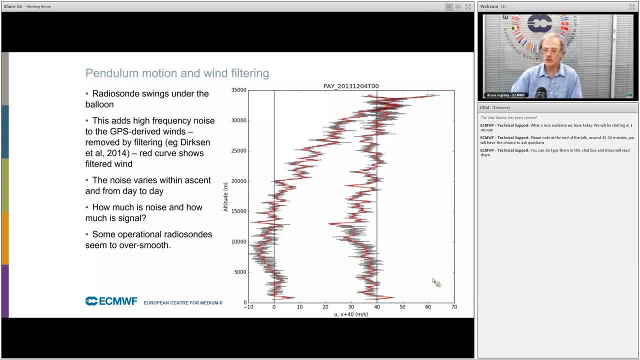 the noise varies at different levels in the vertical. it also varies from day to day and there is a fundamental question: how much is noise and how much is signal? and it's certainly not clear to me from looking at a plot like this and some operational radio sounds. 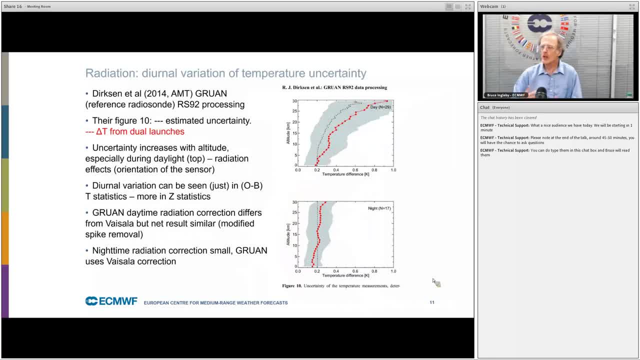 may over smooth the winds. I mentioned the diurnal variation of temperature uncertainty. the top plot here, taken from a paper by Dirksen et al, shows the uncertainty in the day time and the lower plot shows the night time. and you do get a measure of the fact. 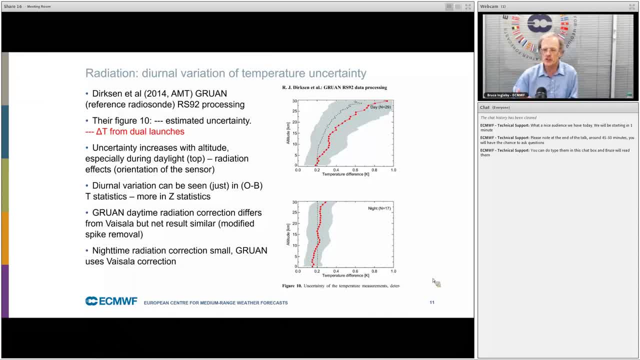 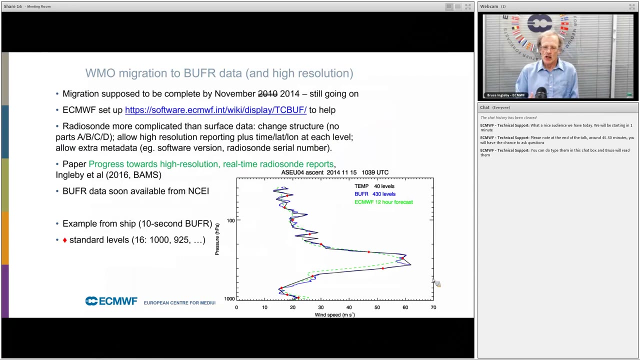 at night time that the uncertainty is more or less constant with height, whereas in the day time it's increasing a lot at the upper levels. this is from the GRUAN, the reference upper air network processing. move on to the next. the transmission of data is coordinated through WMO. 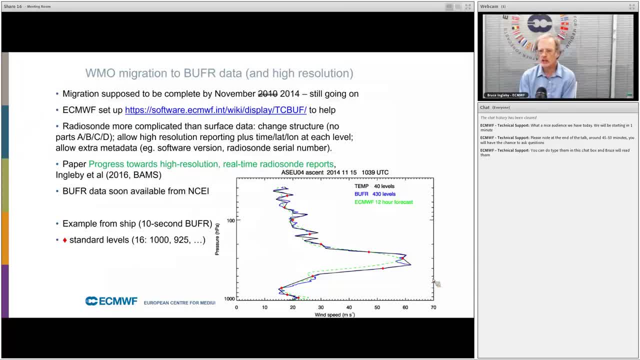 the world meteorological organisation and it used to use alphanumeric codes, notably the TEMP code, and now there is a migration to buffer a binary code which was supposed to be completed some years ago but is not yet complete. ECMWF has been helping and monitoring the process and 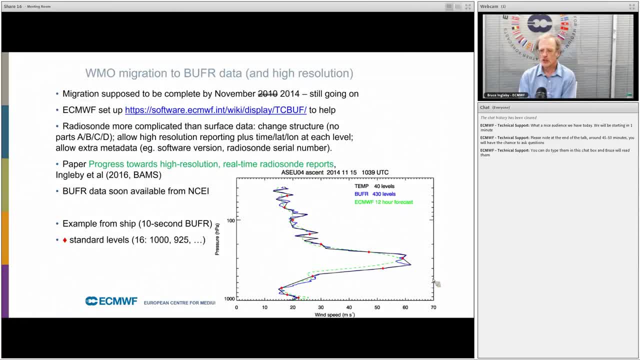 the migration to buffer is more complicated for radiosonde than it is for surface data because there is a change of structure. no longer are there parts A, B, C and D. the whole of the profile should be available in one report and this makes it difficult to simply. 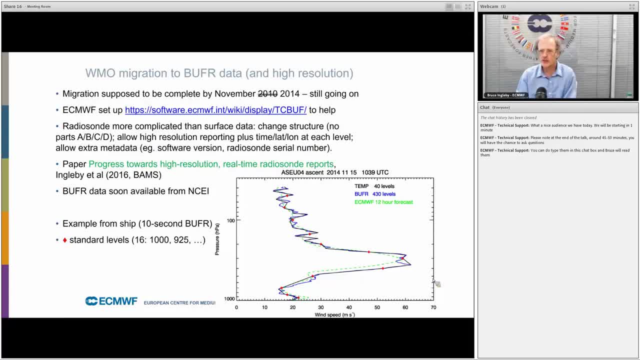 convert from one format to the other. for surface data, conversion does work. for radiosondes, it doesn't really work. there is a paper from 2016 about the process towards high resolution radiosonde reports and the data should be available soon to those not working at. 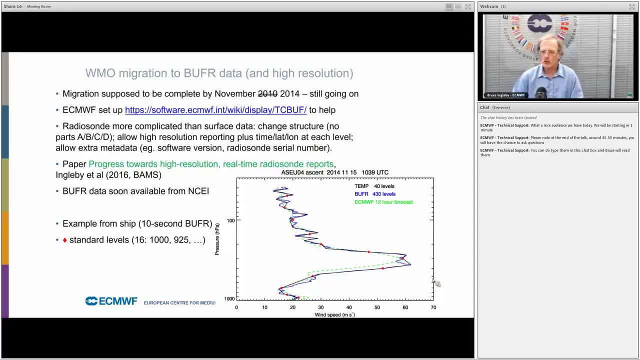 NWP centres. the plot shows an example from a ship with 10 second vertical reporting. so you can see the black line showing the alphanumeric data: 40 levels. this is wind speed, the buffer 400 levels. in this case for some reports we get 4000 or more levels. 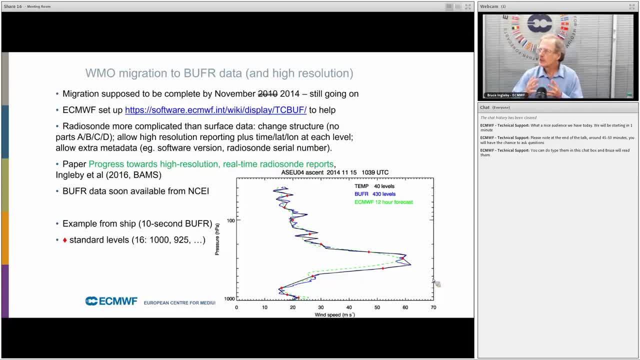 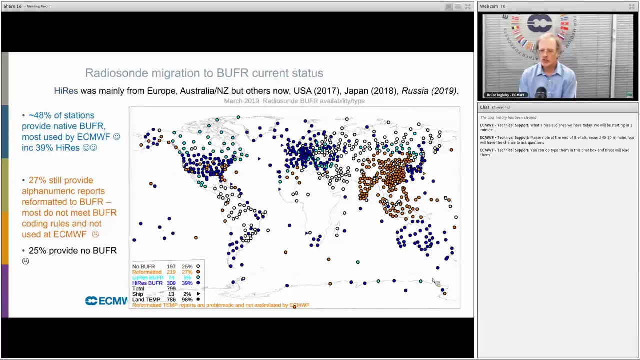 and you can see the extra detail in the buffer and in this case the green dashed line shows the ECMWF background. now the migration is slow but there is progress. 4 or 5 years ago it was mainly Europe and Australia sending high resolution data. over the years, 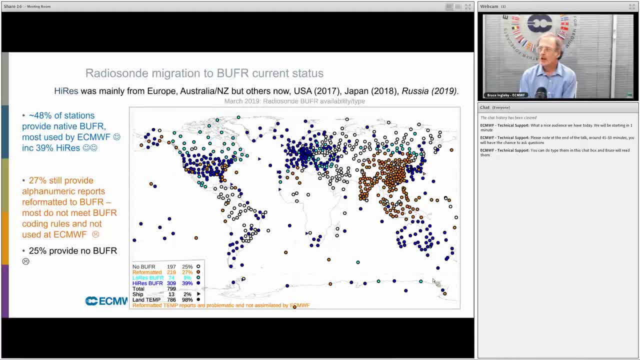 more countries have started sending data, until it's almost 50% of stations sending what we call native buffer. now most, but not all, of the native buffer is high resolution. about a quarter of stations are still providing reports that are converted from alphanumeric, which is not very usable. 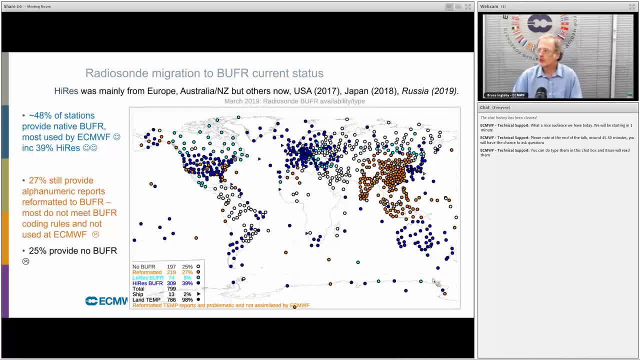 as far as we are concerned, and a quarter provide no buffer, so there is still quite a way to go. one other point on this map is that you see the rather uneven distribution and the particular gaps in Africa, and the coverage there has got somewhat worse in recent years. 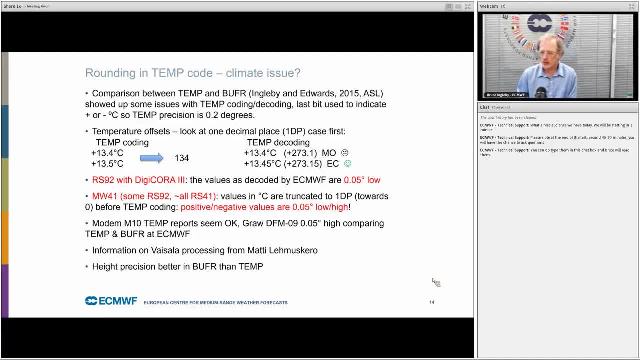 I'm not going to go through this slide but just to mention to anyone that is concerned about very small trends over a climate timescale, you should know that there is some rounding in the old alphanumeric code and I can provide more details of this. so the trends: 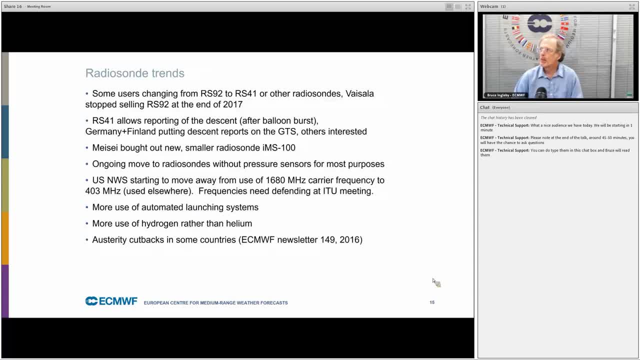 that have been going on over the last few years. the Vaisala RS92 used to be the most widespread radius on. Vaisala has stopped making that and many countries are changing to the newer RS41 or to other radius ons and the new Vaisala software. 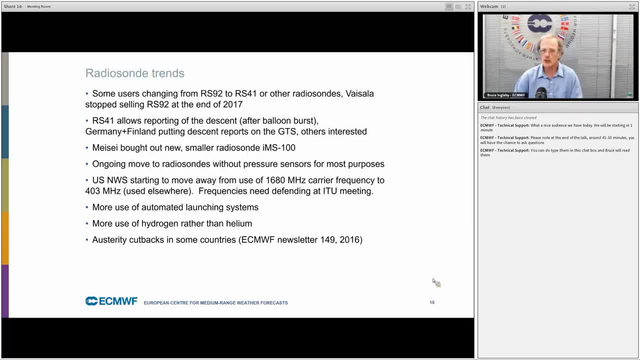 allows reporting of descent data, which I'll say more about later. other manufacturers are also moving to new, smaller radius ons and there is a move towards not using a pressure sensor. the US National Weather Service is going through a big procurement and also changing the downlink frequency. 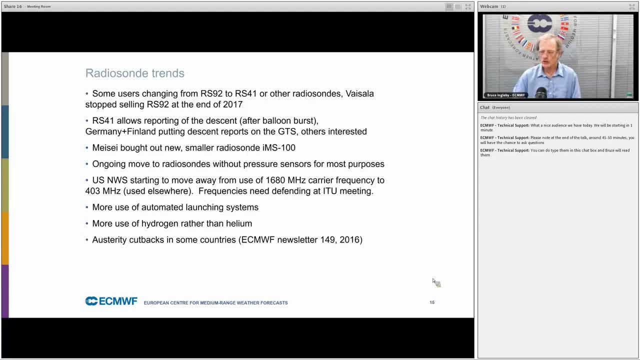 the US and other countries are or will be making more use of automated launching systems, and some stations are changing or changing back to use hydrogen rather than helium. austerity cutbacks in some countries have meant a reduction, sometimes going from two reports a day to one report a day. 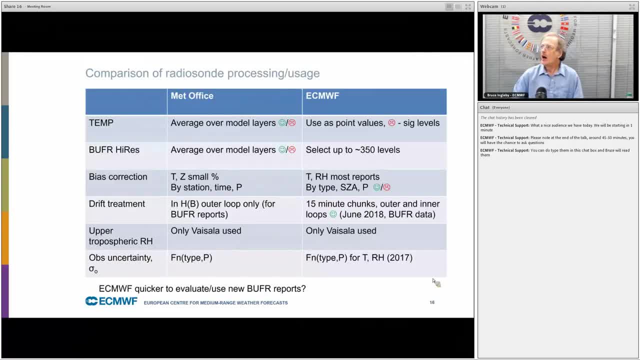 at particular stations and I'll just say a little bit about the processing of data at NWP centres. and this, for comparison shows, summarises what is done at the Met Office and ECMWF. so the alphanumeric data: the Met Office averages that over the model layers ECMWF. 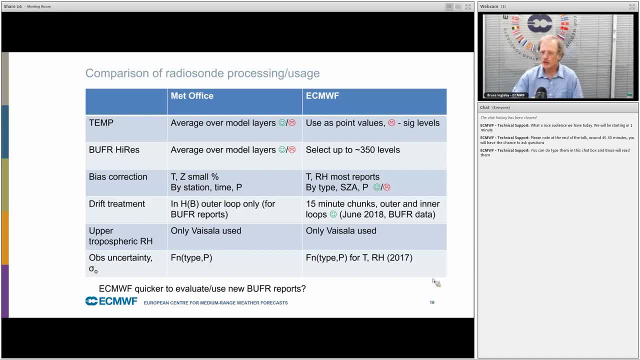 tends to use the whole profile from alphanumeric with the high resolution data. ECMWF selects levels up to about three per model level. both centres do a certain amount of bias: correction of temperature and, in the ECMWF case, humidity. treatment of drift I'll talk about later and the 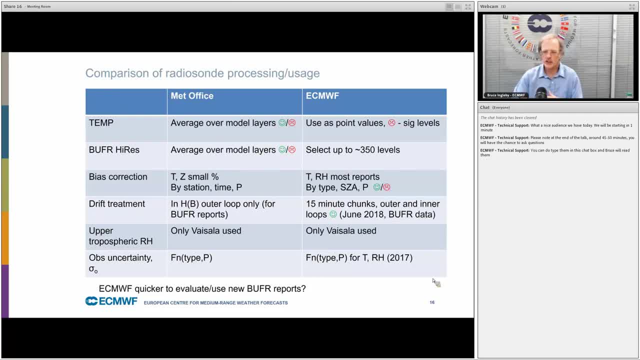 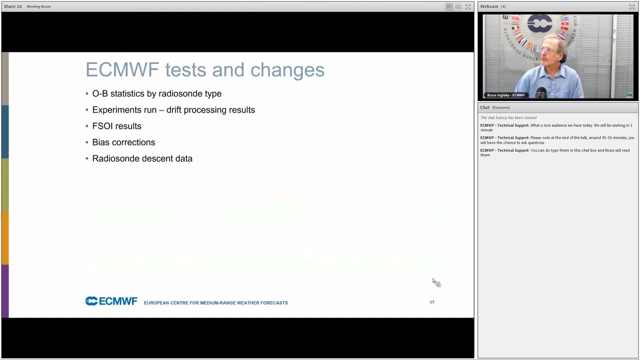 specification of observation uncertainty, which is now a function of radius or type as well as the pressure. so now I'll talk about ECMWF tests and changes. I will show observation minus background statistics by radius or type, and if I say O-B, that means observation minus background or 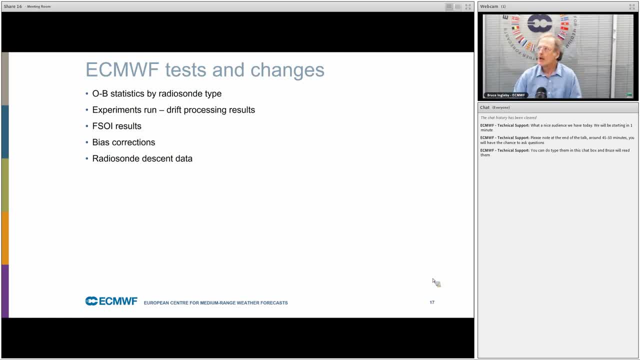 observation minus short range forecast, some of the experiments that we've done, particularly drift processing. I'll explain a bit about FSOI, looking at the impact bias, corrections and descent data. so I've now got a number of slides looking at different radius or types. this is 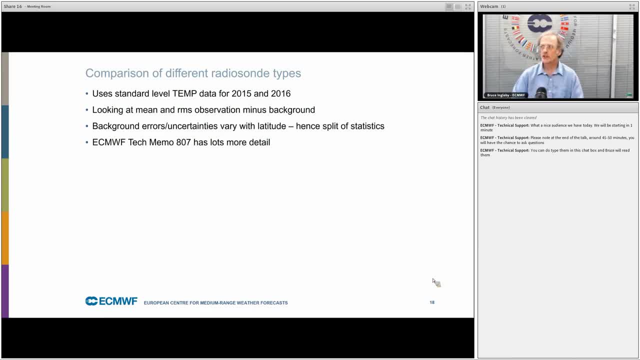 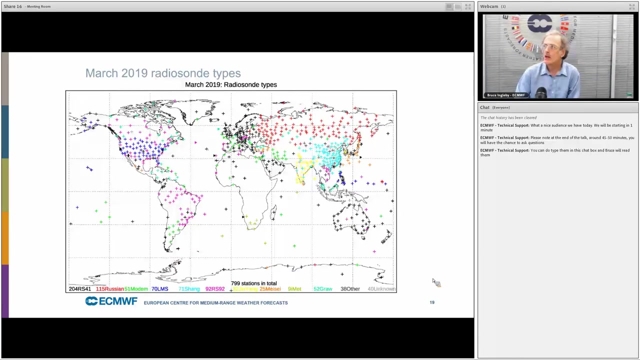 using data from 2015 and 2016 and there is an ECMWF tech memo about this. I'll be showing the mean and RMS, O-B and, but there is variation with latitude of these, so I'm going to show results split by latitude. um, now this. 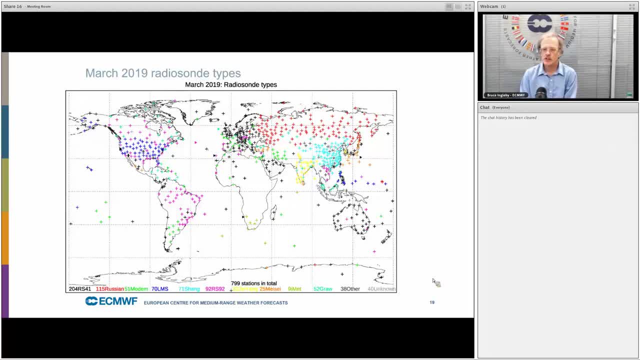 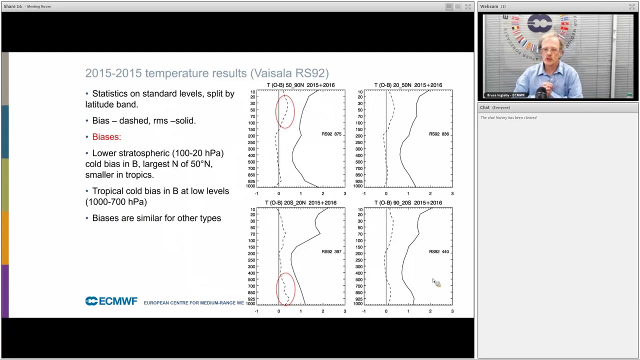 shows the current distribution of radius or types, and the RS41 is currently the most used. if you go back three or four years, many of the stations sending RS41 were sending RS92. I won't go into the other details on this map, so this shows temperature. 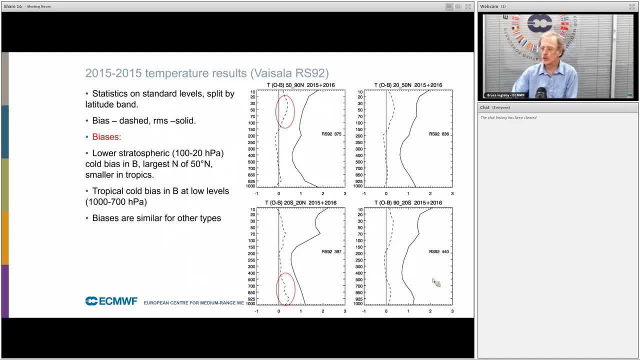 statistics for the RS92, which was the most common radius on that time and also a very good quality radius on um. so there are four latitude bands shown. top left is 50 to 90 north. top right is 20 to 50 north. top bottom left is: 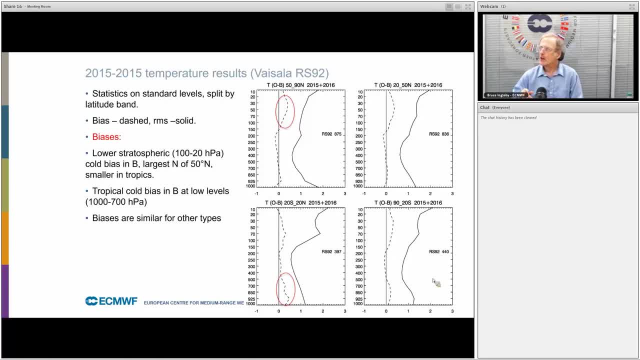 the tropics and bottom right um the bias is shown dashed and the RMS is solid. and I want to point out two aspects of the bias on this um in the extratropics there is some bias in the um in the lower stratosphere and 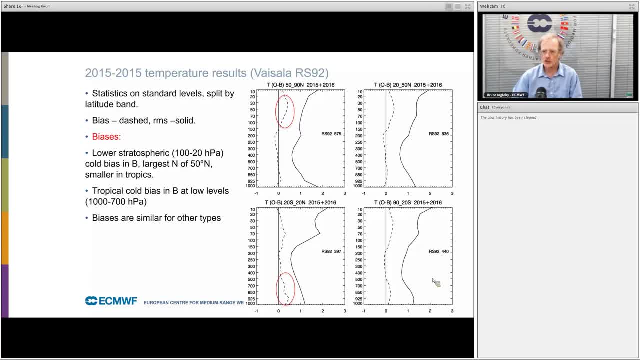 this is largely a problem with CMWF forecast system. uh, and there is also a tropical cold bias in the model at low levels. um, these are the same plots and I'll draw attention to two aspects of the RMS. um, near the surface, in the northern high latitudes. 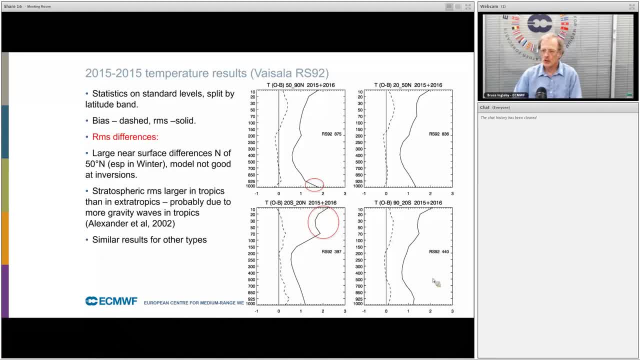 there are some large RMSs. this is particularly at 1000 hPa and this is because over Russia, Alaska and so on you can have very large temperature inversions which the model only partially captures. um in the tropics we see larger stratospheric RMS. 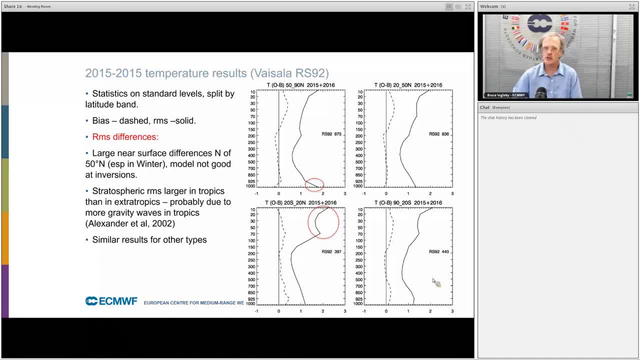 than in the extratropics, and I think this is largely due to there being more gravity waves in the tropics and there tends to be a bit of a peak at the tropopause level, which is obviously varying with latitude. and now I'm adding all the different radius on types. 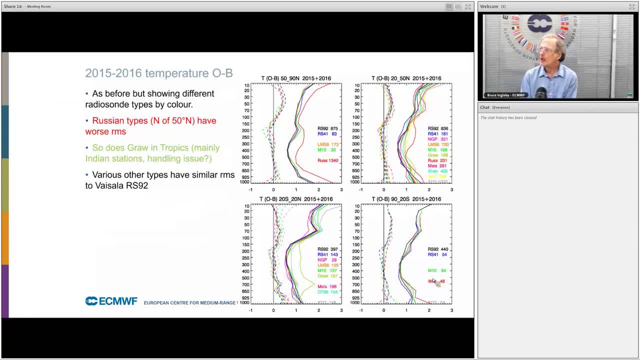 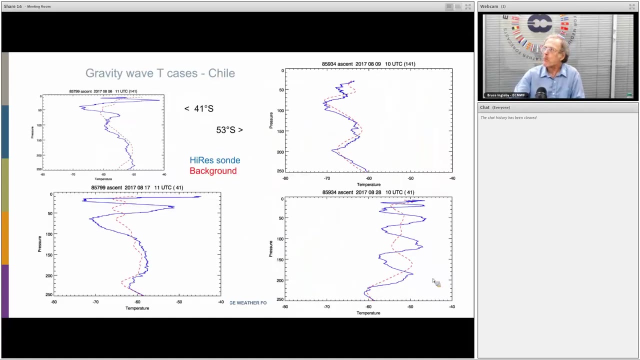 and um. you can see they've got features in common and there are also one or two outliers. the Russian radius on the red line have somewhat worse RMS um. I mentioned gravity waves and this is showing examples from Chile. in the temperature you can see them in the winds as well at times. 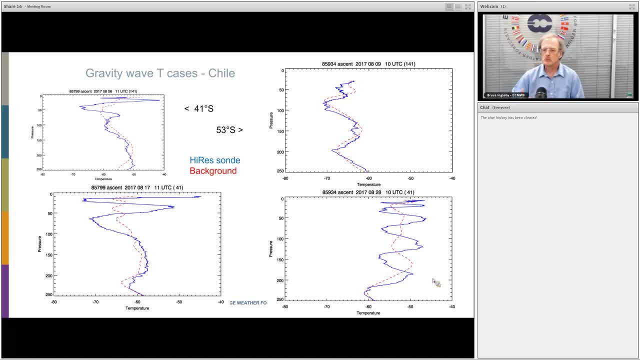 and this is four different cases. so solid line is the radius on red, dashed line is the background, and the remarkable thing here is that at times, like the top right case, the background does a very good job and in some of the other cases it does a very poor job. 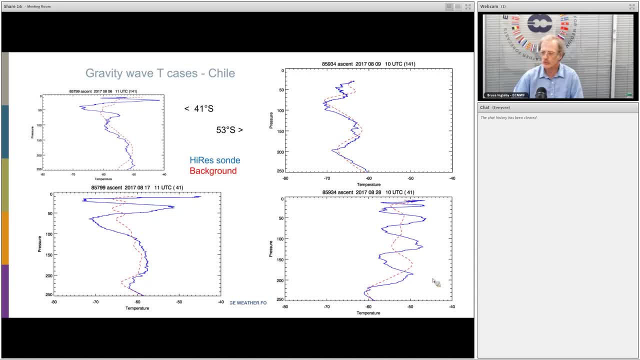 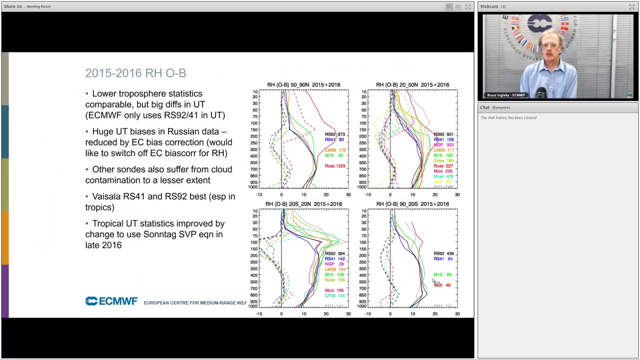 of representing the gravity waves or other waves, and this is partly to do with the vertical scale of the wave, as you would expect. um, these are similar plots for relative humidity. um now in the lower troposphere, up to about 400 hectopascals. the statistics. 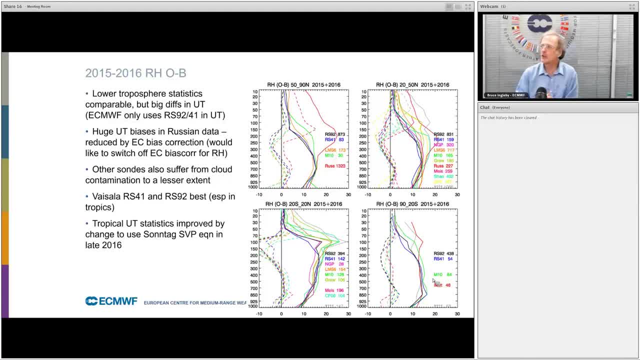 are fairly similar between the different radius on types um, but at upper levels there is a lot more variation and there are quite large biases, the Russian data in particular. they are particularly susceptible to contamination after going through cloud um. yeah, in general, the Vaisala radius on: 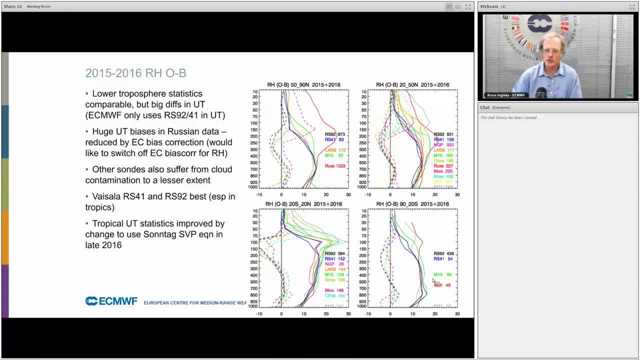 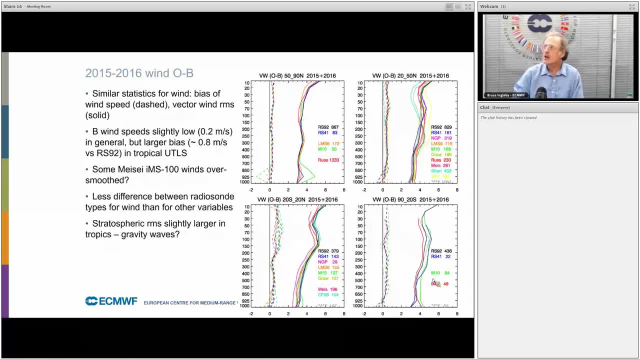 do best for upper tropospheric relative humidity. this is most obvious in the tropics. ok, and this is a similar plot, but for the wind statistics, um, the solid line in this case shows a vector wind rms and the dashed line shows a wind speed bias. the 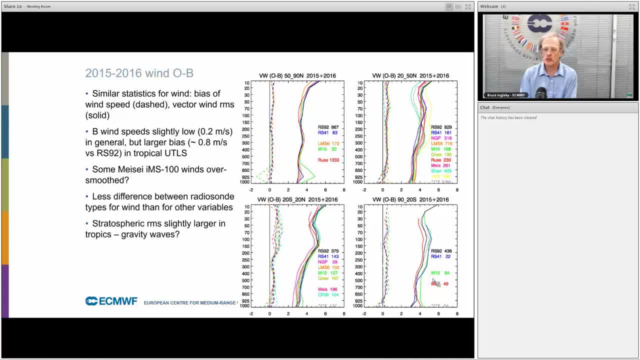 background wind speeds are slightly low compared to the observed ones um the rms's are quite comparable between the different radius on types. so when ECMWF put in different radiation errors for different radius on types for temperature and humidity, we decided to leave them all the same for wind. 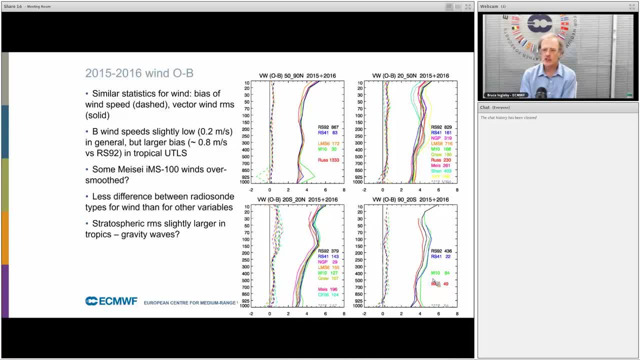 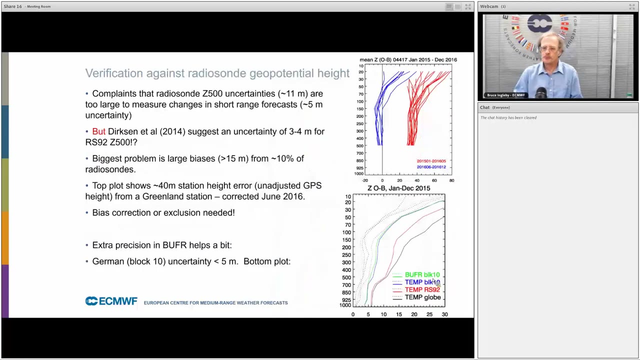 and in some cases there is a suggestion that there is over smoothing of the winds, as I mentioned, and there is in the stratosphere. there are somewhat larger differences in the tropics than in extra tropics and gravity waves um geopotential height we don't. 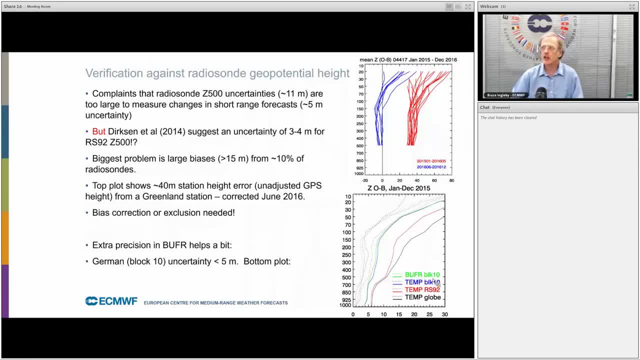 assimilate, but it is used for verification and in the last five years or so there has been a number of complaints that radius on um heights, particularly at 500 hectopascals, which is a sort of standard level, are not accurate enough to use for short range. 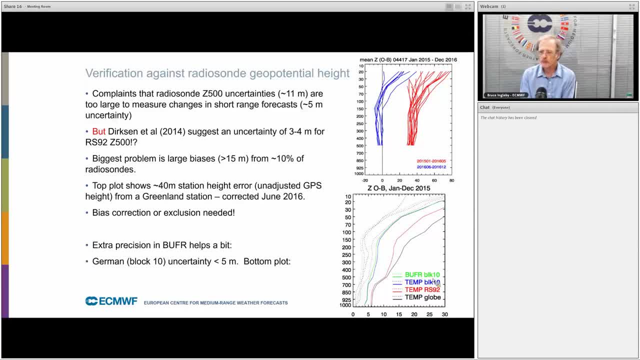 verification and I have looked at this issue and I think the main problem is that a fraction of radius on perhaps 10% have relatively large biases in their heights and in most cases this is due to a station height error, either in total or to the height. 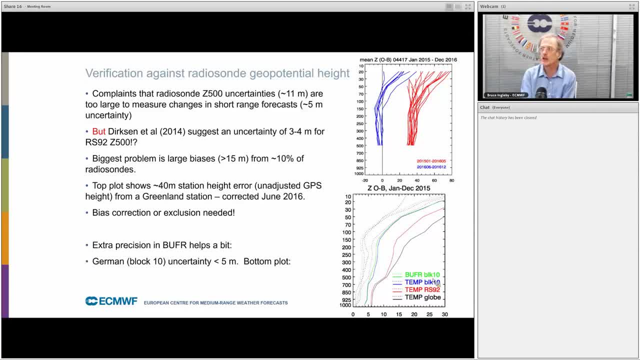 assumed for the pressure sensor and we came across one case for a station in Greenland- the plot at the top right- which had a height bias of 40 metres and it did, which was to do with using an unadjusted GPS height. it wasn't adjusted to mean sea level. 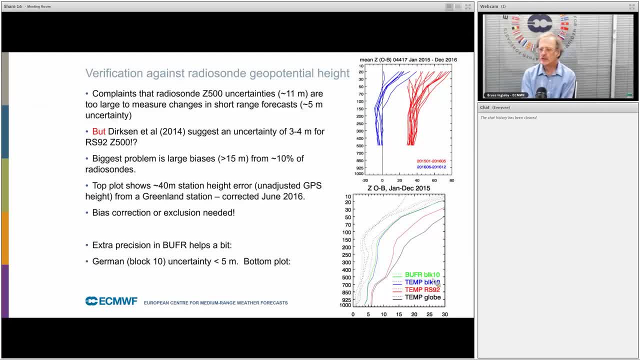 and we contacted the operator and they fixed it and after that it agreed much better with the ECMWF forecast. so the blue lines the months after the change show much better agreement with the ECMWF forecast system. one other aspect is that the extra precision in buffer does help somewhat. 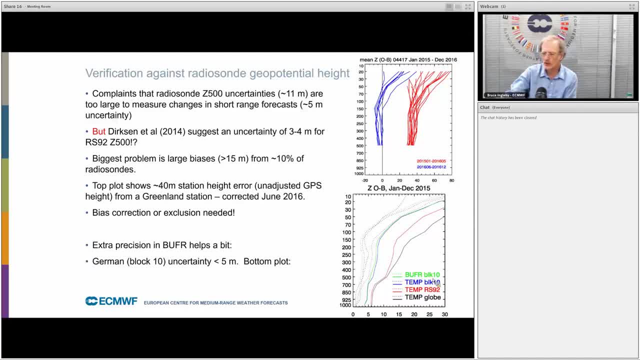 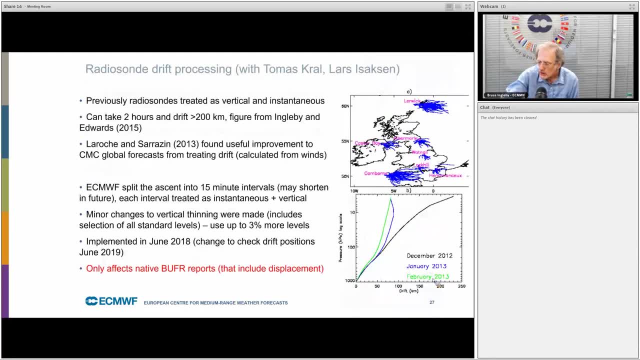 with for height and the differences with the model height. right now I'm going to talk about radius on drift processing um. in the early days of forecasting and until quite recently, most centres treated radius on as vertical and instantaneous, and they're not um. it takes something like: two hours for a balloon to reach 35 kilometres and during that time it can drift 200 kilometres or more. um it, the amount of drift does vary a lot from case to case, month to month. as the bottom plot shows, it does tend to be further in winter. 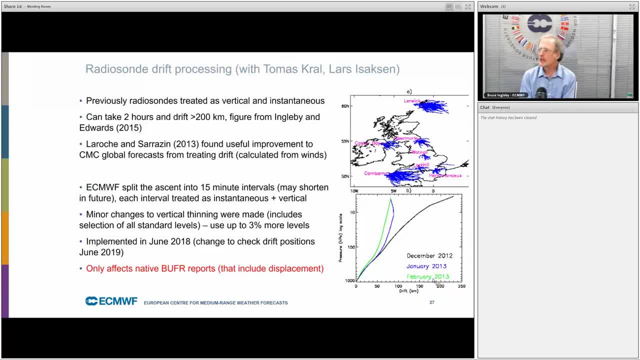 there's some nice work done in Canada by the Russian Sarazan about treatment of drift and in 2018, ECMWF implemented treatment of drift in our NWP system. for technical reasons, we split the ascent into 15 minute intervals and within each interval we treat it. 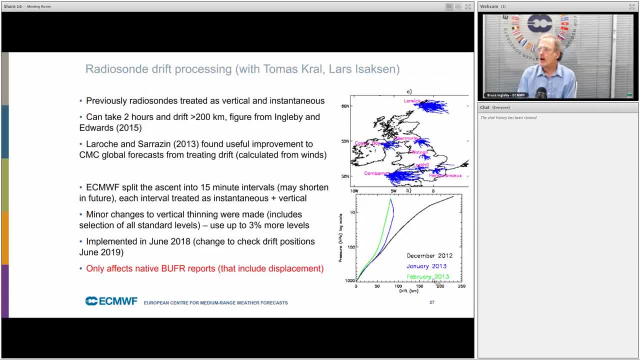 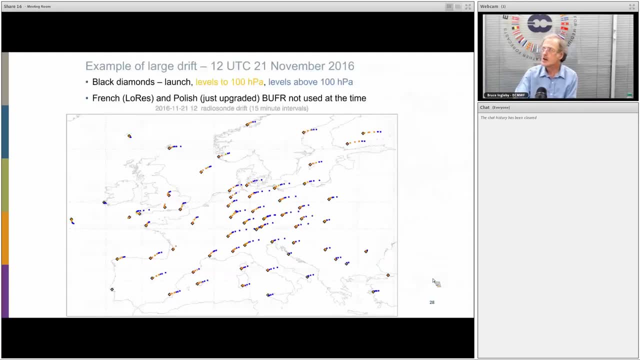 as vertical and instantaneous um um, and in a few months time we're going to add a check on the drift positions, because occasionally there are errors in those and this just shows another example of a fairly large drift and including a case over 300 kilometres. now this does improve. 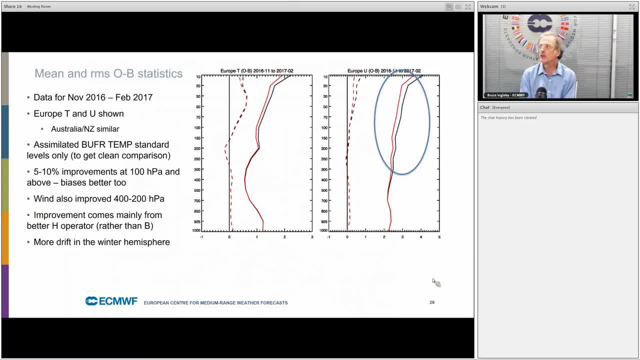 the fit between the observation and the background. um. this shows temperature left and the U wind on the right. the black line is without drift taken into account and the red line is with drift taken into account and um you can see improvements of between 5 and 10 percent. 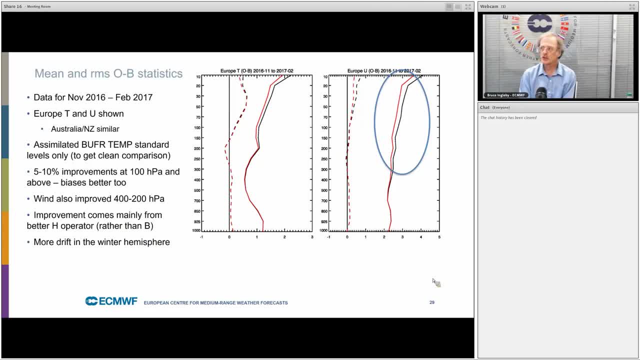 in the RMS fit at 100 hectopascals and above and, slightly more surprisingly, the wind bias has improved a little bit as well. the improvement does come largely from the better observation operator and, as I said, we get more drift in the winter hemisphere um this. 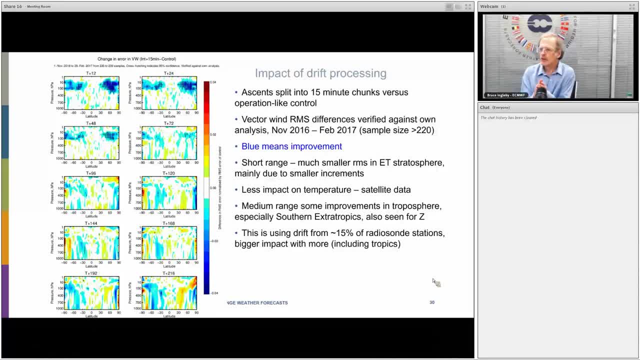 uh shows the verification of forecast at different forecast range against the analysis. this is for vector wind and blue. uh height or pressure against latitude and the blue indicates that there is a better fit and you can see that certainly at the shorter ranges, out to two or three days. 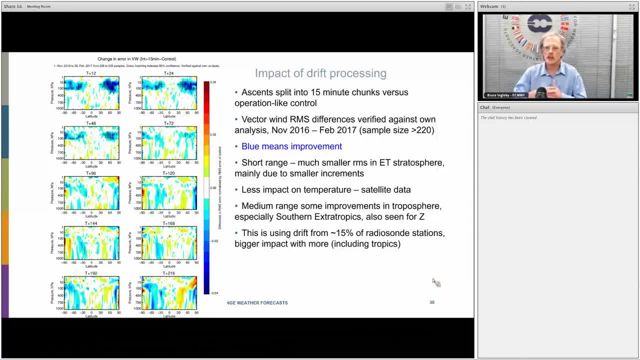 um. it's mainly blue in the lower stratosphere. so we do see some improvements in the forecasts at relatively short range. for some reason the improvement seemed more marked in the southern national tropics and the northern national tropics. this particular example was done um two or three years ago. 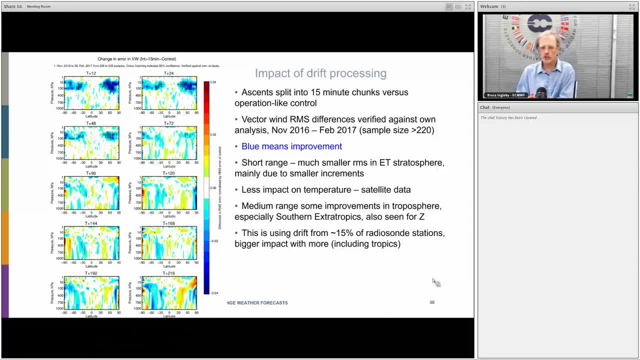 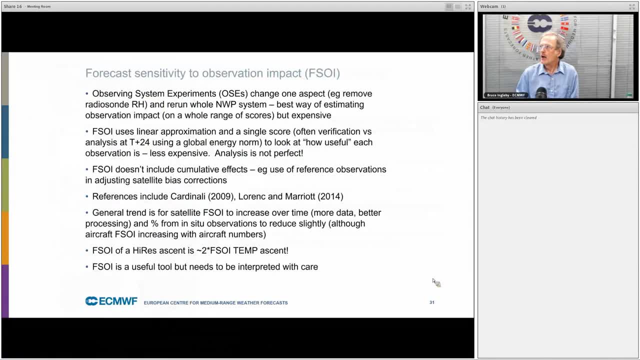 and there are more radius arms giving us drift now, so we would hope to see a bigger impact. now. some of you have heard of forecast sensitivity to observation impact, or FSOI. it's one way of looking at the impact of observations. in some sense, the ideal is. 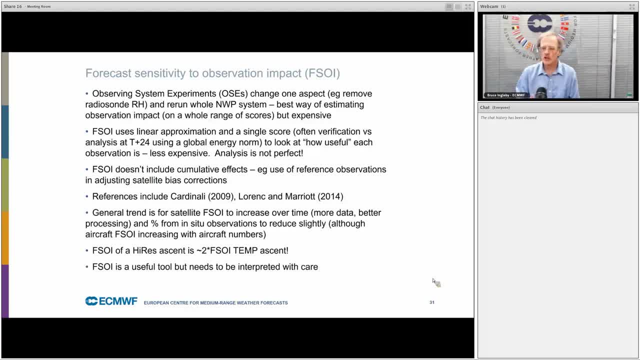 observing system experiments, which is to change one aspect of the observing system and rerun the whole NWP system and then look at the different scores. um, but that is really quite expensive, particularly if you want to take out various different observation types. FSOI uses a linear. 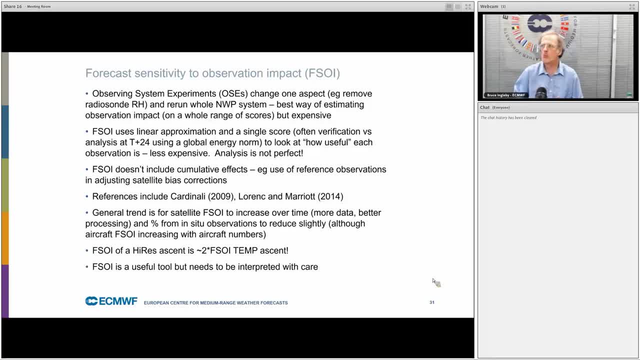 approximation and a single score um, often verification against analysis at T plus 24 using a global energy norm and there are various approximations in this. it also doesn't include cumulative effects such as the use of radius arms in helping to anchor or provide bias corrections within an NWP system. 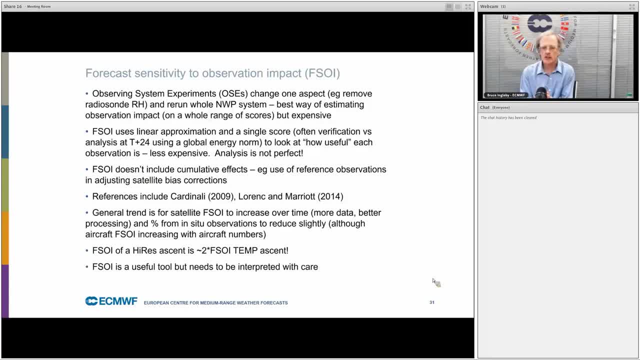 now over time satellite FSOI is tending to increase um more data, better processing, and so there is some decrease in the FSOI of conventional observations. for aircraft this is offset by increased aircraft numbers, but we do see some evidence that the FSOI of a high 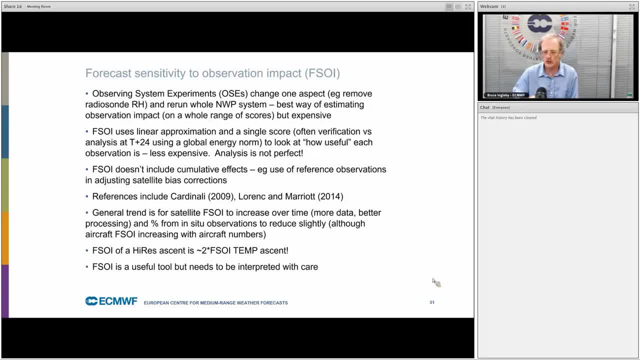 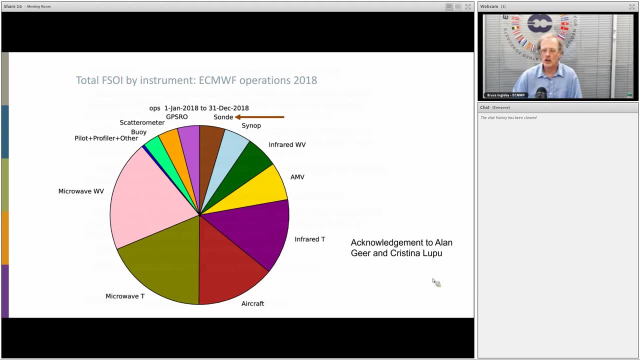 resolution ascent is about twice that of a low resolution ascent, and this is a useful tool, but it needs to be interpreted with care. and this shows our average FSOI for last year, 2018, and the brown segment shows the radius on impact using this measure. 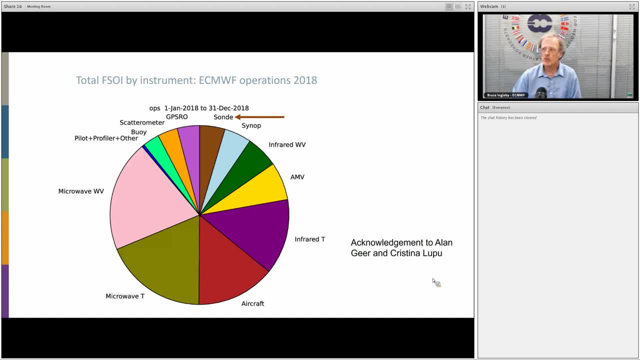 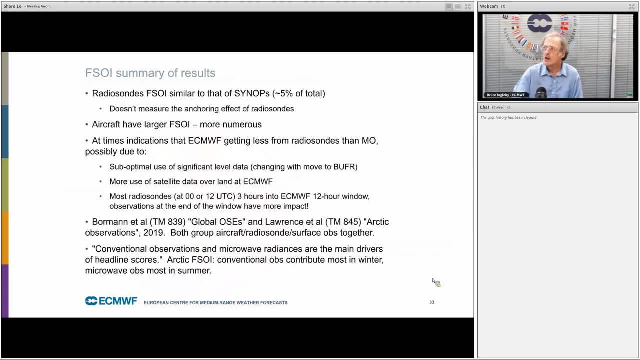 and it's similar in magnitude to the Sinop impact, rather less than aircraft, and you can see big chunks from microwave and infrared satellite data. um, I have said some of this, um, at times there have been indications that ECMWF is getting less impact from radius arms than the Met Office. 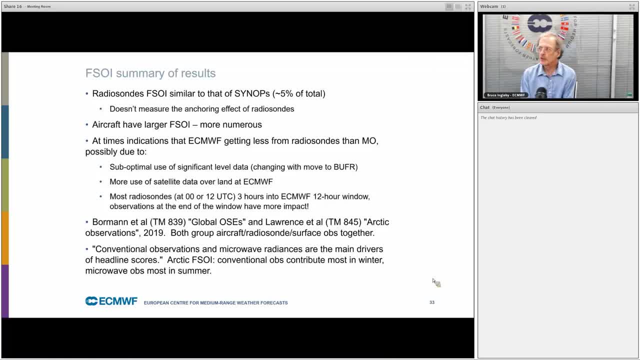 possibly due to suboptimal use of significant level data um. that problem is reducing as we move to buffer data, possibly more use of satellite data at ECMWF um and also a technical reason to do with the ECMWF 12 hour windows. there have been two recent ECMWF tech. 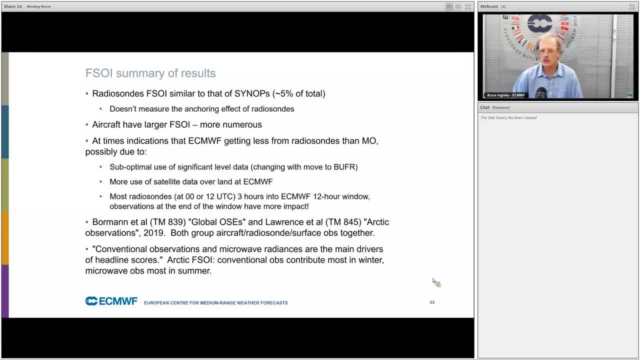 memos by Bormann et al and Lawrence et al which you might want to look at if you're interested in the impact of data. they haven't separated out radius arms, but they've combined it, combined them with surface and aircraft data and found that conventional. 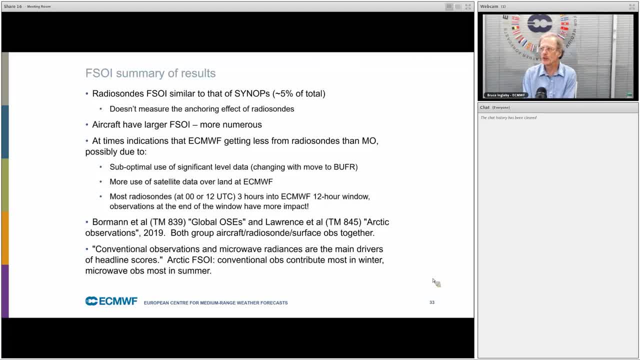 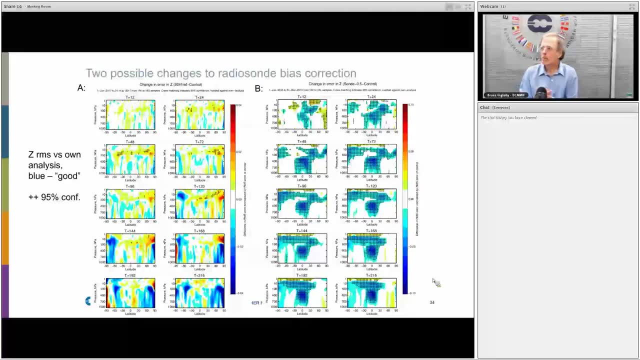 observations are still very important and particularly in the Arctic in winter, conventional observations seem to be the most important source. now this again shows two changes to radius arm bias treatment A and B. I'll go into the details in a moment. this is measured against analysis height. verification against analysis height. 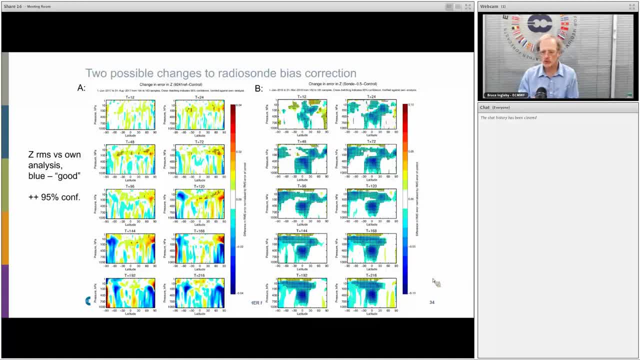 and again, in general terms, blue is smaller differences, which is generally a good thing. and the left plot. you can see a mixture, um, probably marginally better. the right plot. you might think, oh, this is a wonderful change um, and then I'll tell you we made change A and not change B. 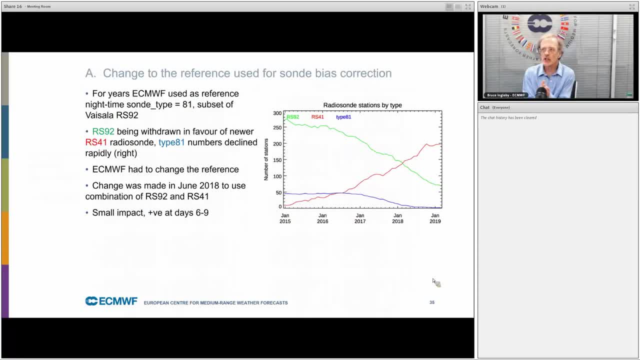 but change A was a change to the reference used for the radius arm bias correction. for many years the system used night time autosonde RS92 as a reference and we realised that the numbers of the reference observations were declining quite strongly, so we had to change things. 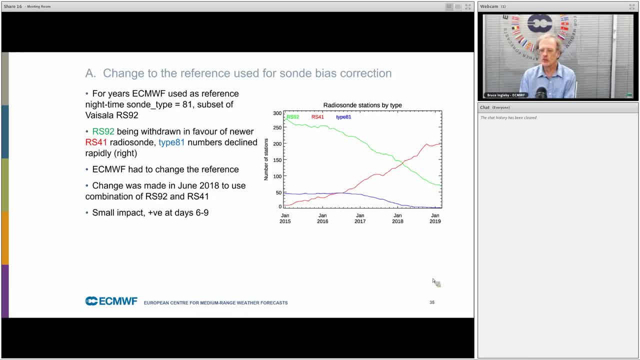 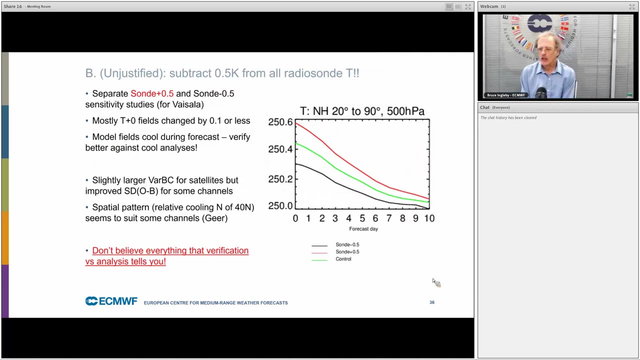 and we changed to use the average of RS92 and RS41. the change was made last year and the impact is relatively small, but we think if we hadn't made that, our system would have been getting worse by now. now, the other change was a sensitivity test. 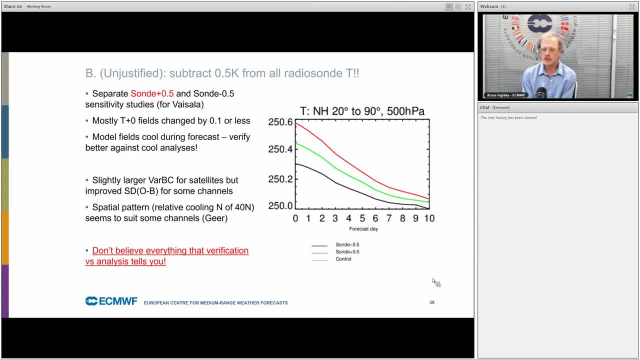 uh, I ran two tests, one adding half a degree to all radius arm temperatures and the other subtracting half a degree from all radius arm temperatures. um, the analysis fields didn't change that much, but it was enough to make a difference to the verification against analysis and this. 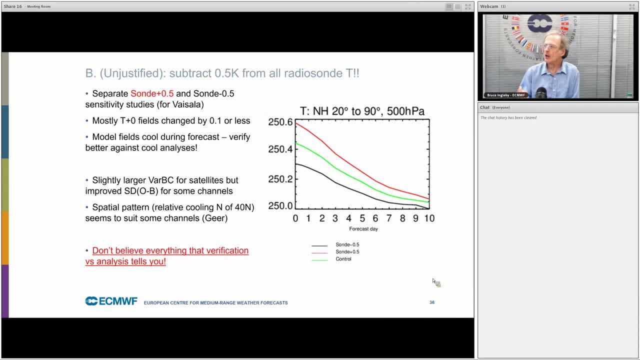 plot shows one example: um one level, one latitude band, that the. because of climate biases in the system, the model is cooling as it goes into the forecast. and um the if you subtract, if you make the radius arms cooler, then that cooling is reduced. but this doesn't mean 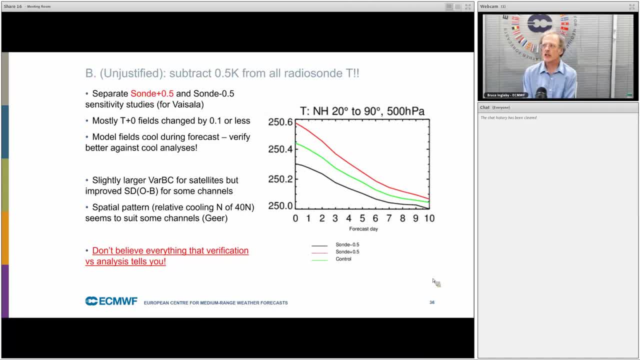 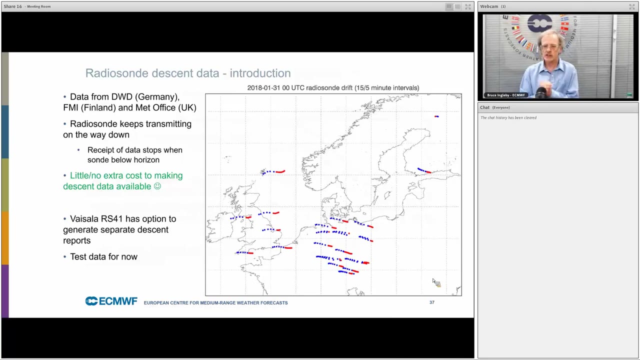 that the analysis or forecast are better. this is just a a warning that with with all sorts of verification, you have to be a bit careful and look at different measures. radius on descent data: this is the last main topic and with radius arms, what goes up has to come down. 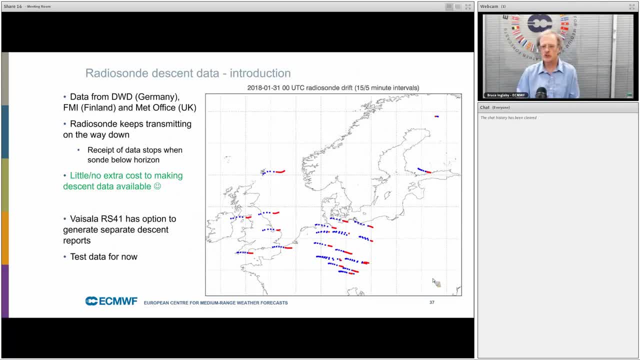 and they can come down in inconvenient places. I've heard stories of them coming down on roads. then the road is closed. you get traffic queuing up until the police have checked that it's nothing dangerous anyway. right these? this map shows data where we've got decent data. 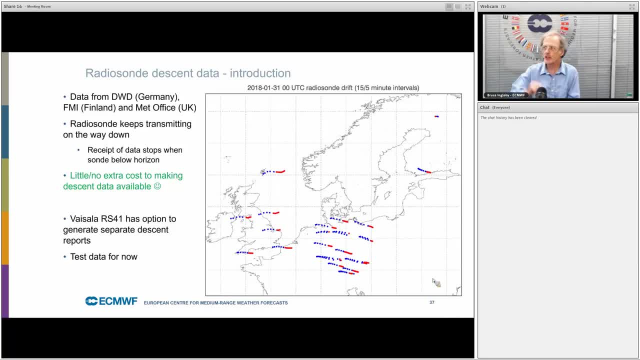 so the ascent is the blue dots shown every 15 minutes and the descent is the red dots shown every 5 minutes. data from Germany, Finland and the UK. the radius arm keeps transmitting on the way down um and the station can continue to receive the data until the radius arm goes below the horizon. 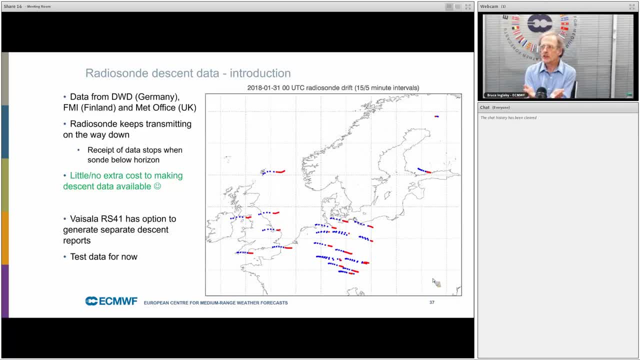 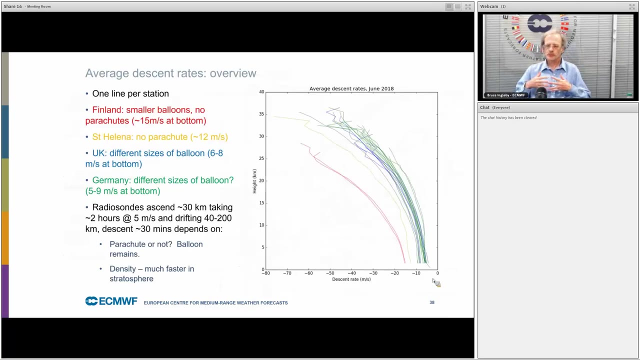 and one of the obvious advantages: there's little or no extra cost to making the descent data um. for now, this is RS41 data and it is still at the test stage um the. to understand what's going on, we do need to look at the descent rates. 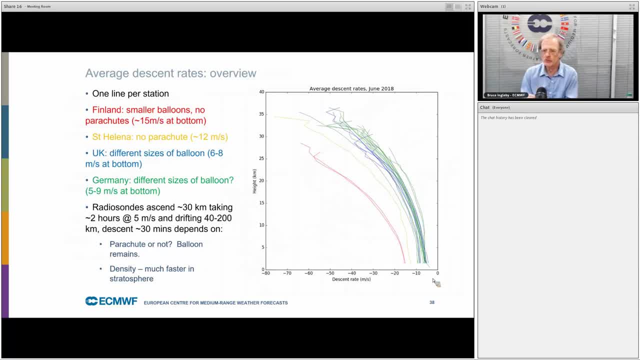 and this plot shows descent rates for individual stations averaged over a particular month. one line per station. now the red lines are for Finnish stations. um. Finland uses smaller balloons, so they don't go quite as high, and they're not using parachutes, so they fall quicker. um. 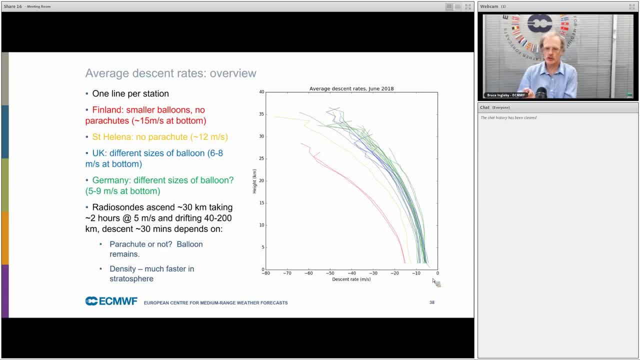 the green and the blue plots show data for German and UK stations uh, both of which use parachutes, so these fall slower and they're using mostly using bigger balloons so that they go somewhat higher in the atmosphere, so that the radius arm they ascend usually between 30 and 35. 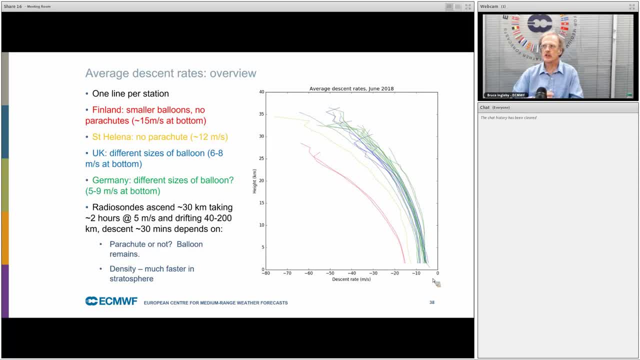 kilometers, taking about two hours, going up at about five meters per second. um, they tend to fall down in something like 30 minutes, but it does vary quite a lot depending on whether it's a parachute or not. and the balloon size makes a difference because it's often falling with the 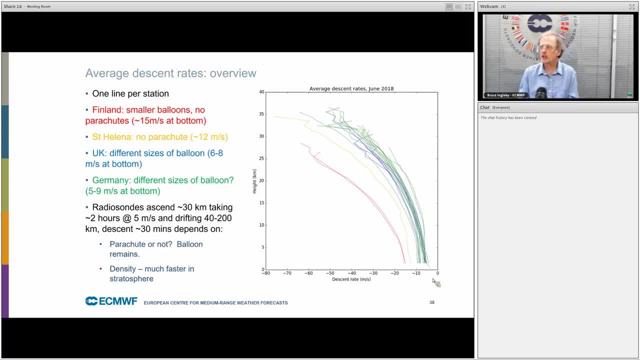 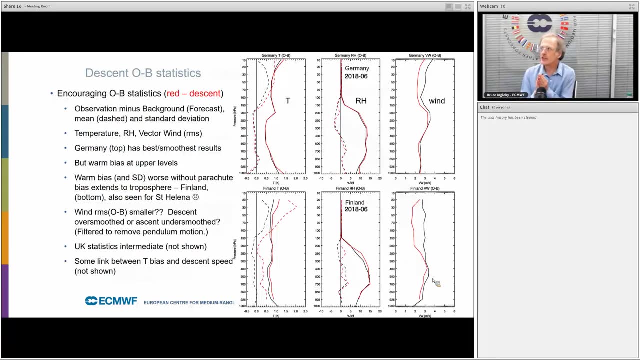 remnants of the balloon and more weight makes it fall faster, and the faster speed in the stratosphere is because the air is less dense. there and right. this is observation, minus background statistics for ascent data in black and descent data in red. uh, german stations on top and the 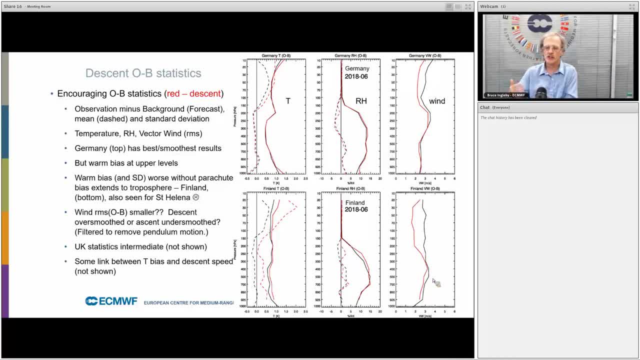 finnish stations on the bottom uk results tend to be somewhat intermediate. the, um, and if we look at the german data top line first, the surprising, perhaps um and encouraging result is that the statistics are fairly similar in general, um, so it does look as if the descent data might. 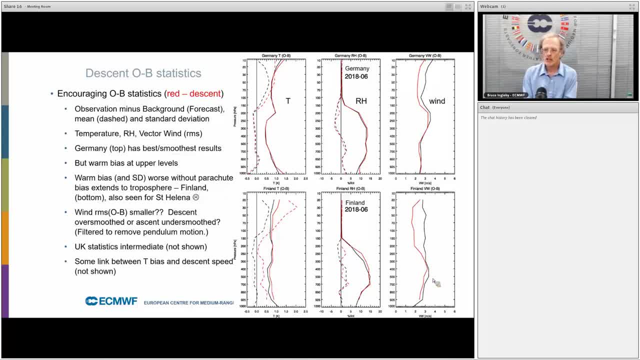 well be usable. um at upper levels. there's a difference in temperature bias. the rh is surprisingly similar for winds. the um fall rate, the descent rms, is smaller than the ascent rms, which was a surprise um for finland. we can see that there's a bigger temperature bias for the. 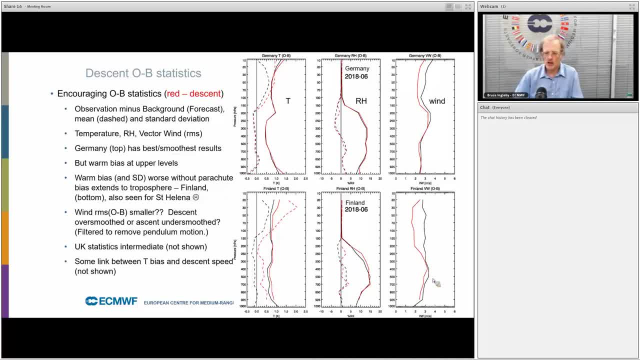 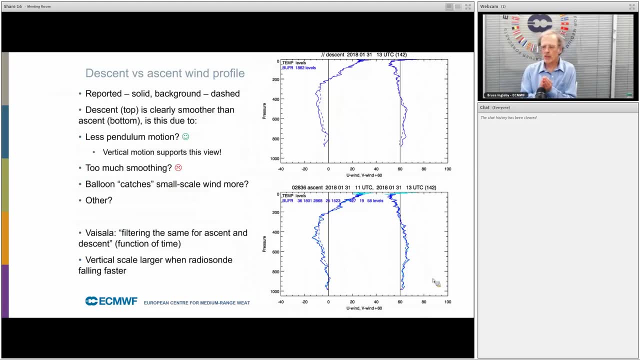 descent data. it does seem to be linked to the faster descent rate. um, um, and just to look a bit more closely at the winds, the top plot shows a descent and the bottom plot shows an ascent for the same radius on there's again, the solid line is: 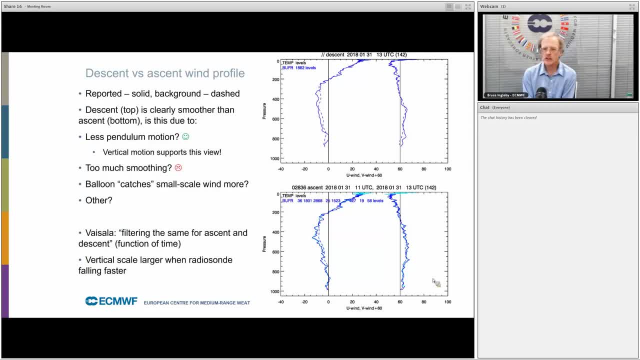 the reported data and you can see that the descent is winds are somewhat smoother than the ascent winds. and is this due to less pendulum motion? there is at least some evidence to back this up. it could also be due to too much smoothing of the descent data. 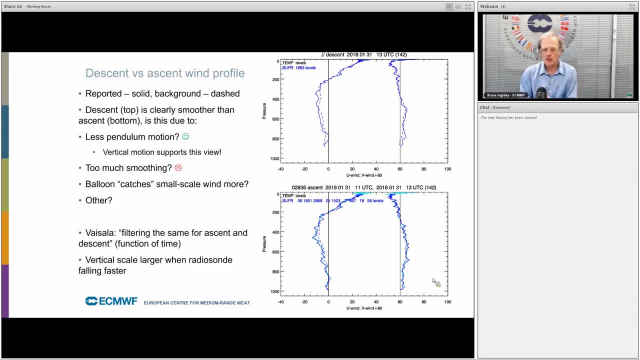 the filtering is the same for the ascent and the descent, as Vaisala tell us. um well, it's the same as a function of time. but because it's falling more fast, then the effective length scales of the smoothing will be greater for the descent data. so I'll 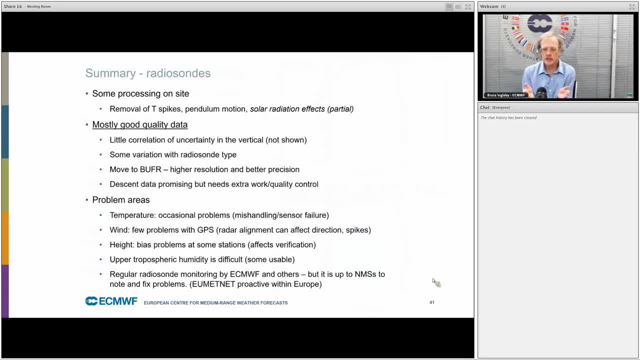 summarise now: um, there is some processing on site- removal of temperature spikes, smoothing out pendulum motion and trying to reduce solar radiation effects- which is only partially successful. um, and this is so what we see is process data, a lot more process than, say, a temperature from a Stevenson screen. 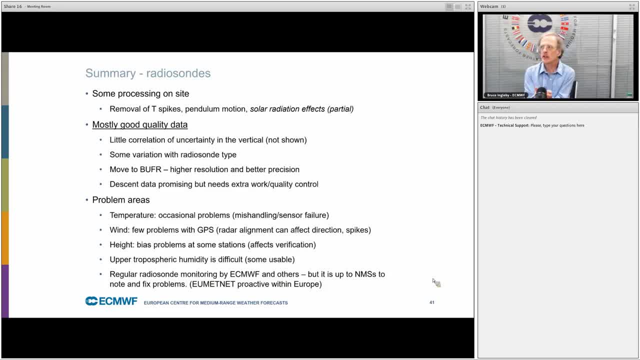 it's mostly good quality data. um. there's little correlation of the errors in the vertical. there is some variation with radius. on type, there's a move to binary data. higher vertical resolution, better precision and descent data is under test. um. there are some problem areas. temperatures: mostly good. there are. 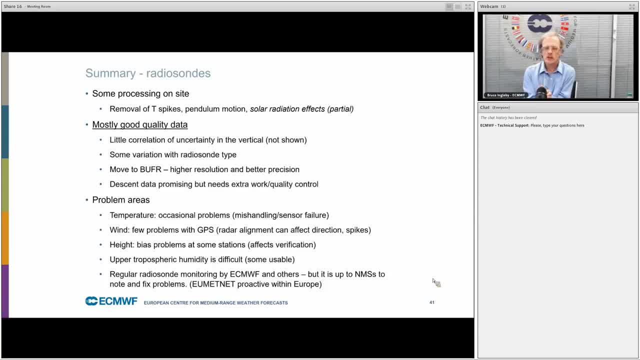 occasional problems. wind GPS results are generally pretty good. there can be more problems with sites using radar height. I mentioned bias problems at some stations. um I mentioned that upper tropospheric humidity is a difficult variable to measure. the best radius ons are usable in the upper troposphere. 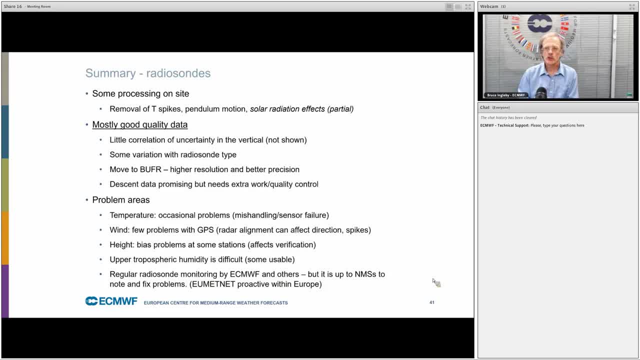 ECMWF does regular radius on monitoring um and we provide the information within Europe by UMetNet um. it is available more widely but once we find a problem it is up to the National Met Services to try and find the route and correct the problem. um NWP. 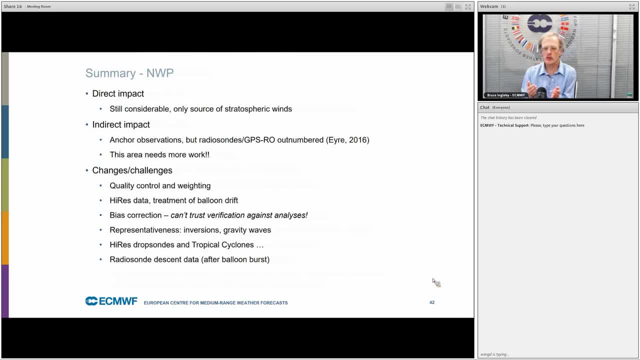 um. there is both direct impact of the radius ons, uh, which is still well worthwhile, and they're more or less the only source of stratospheric wind, say they provide full profiles, as I mentioned. there's an indirect impact, uh. they're used to anchor um the NWP system. 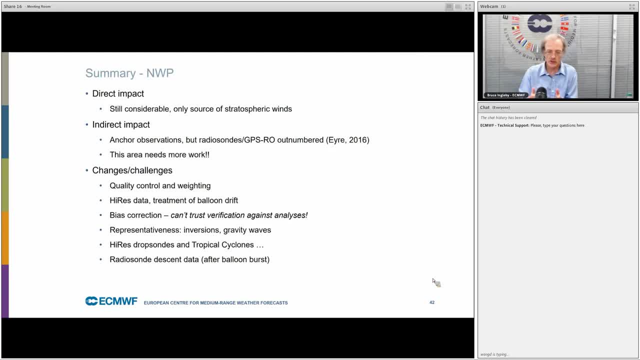 and the satellites bias corrections a lot of, along with GPSRO. um that there is something of an issue in that um. you want a large, a good proportion of anchor observations and in general that proportion is decreasing over time and there's plenty more work could be done on this. 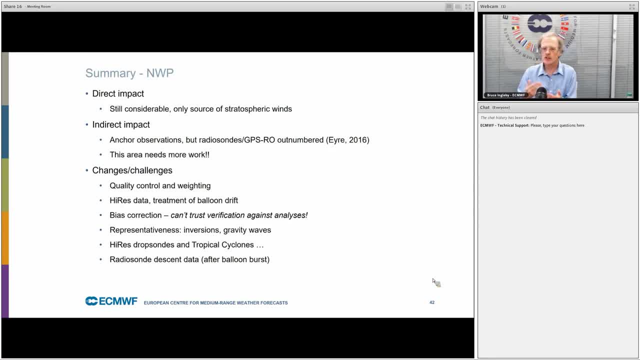 anchoring and bias correction, changes and challenges, quality control and weighting of the observations, treatment of high resolution data, treatment of balloon drift, bias correction, uh representativeness and I'm at the moment I'm doing some work on high resolution dropsondes and tropical cyclones. 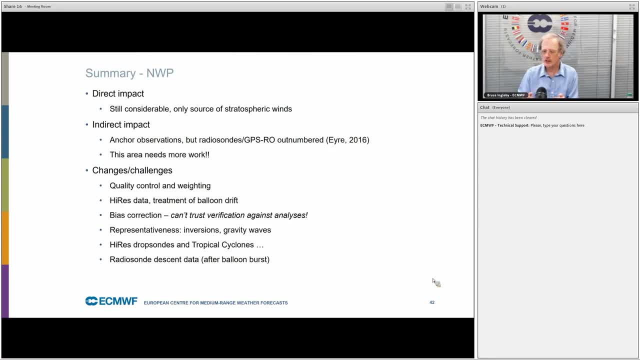 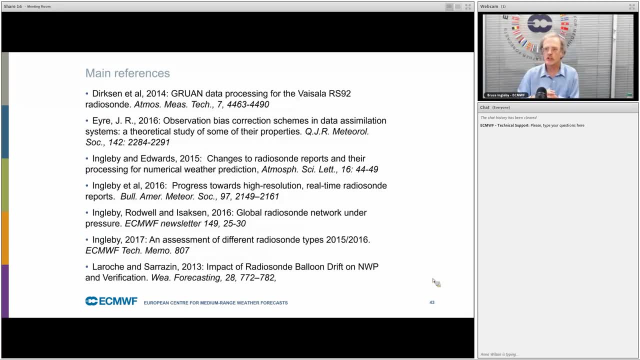 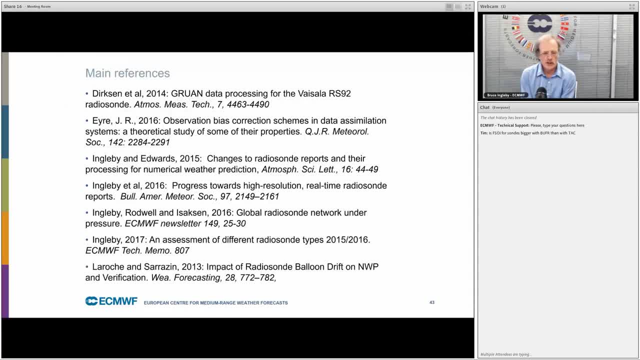 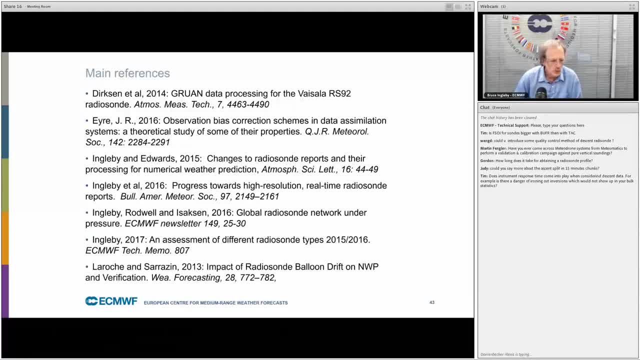 A question from Martin Fengler: have I come across meteodrome systems? and the short answer is no, I haven't. You can send me information if you want. How long does it take for obtaining a radius on profile? It takes about two hours to go up. 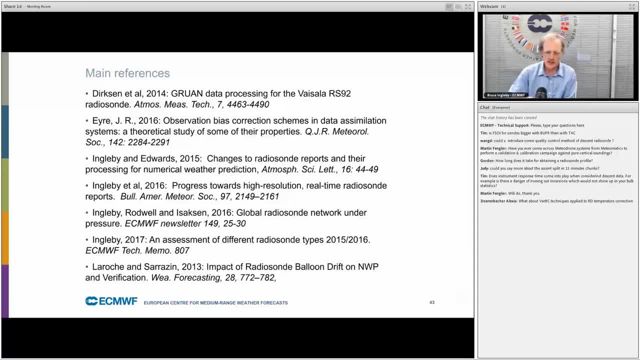 They do tend to send data when it gets to 500 hectopascals, sorry, when it gets to 100 hectopascals. There are discussions going on as to whether it would be good to send data from lower in the profile. that there's sort of technical issues to sort. 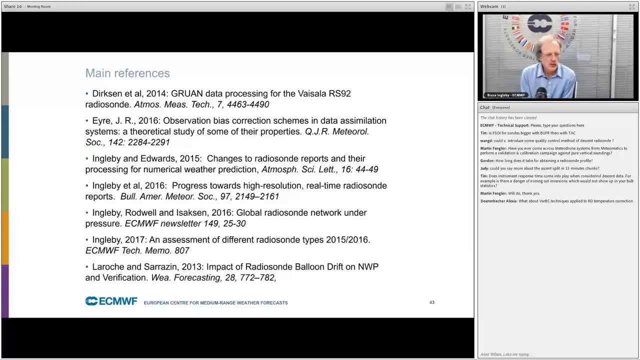 out before that is done. Could I say more about the ascent split into 15-minute chunks? Well, this is the solution that ECMWF has adopted, partly to fit in with our existing system, and if we treated thousands of levels from a particular radius on it? 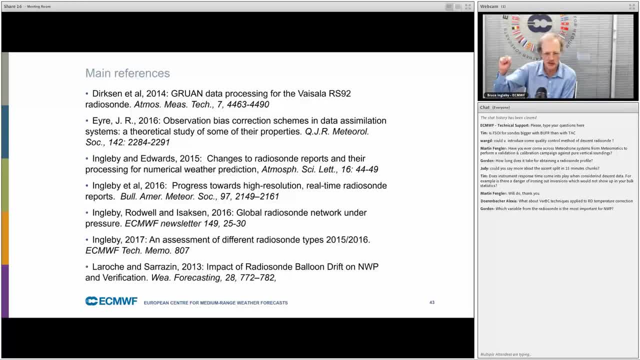 becomes quite inefficient because we would then have a complete background profile for each of them. So it's an efficiency thing, but we may reduce that 15 minutes at some point. Does instrument response time come into play when considering descent data? There might be. 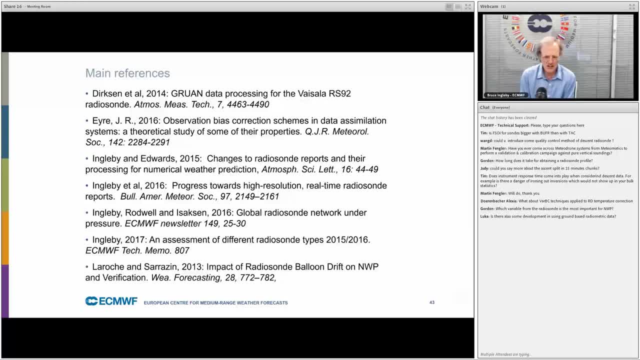 I don't think it's a big issue, but it's one thing to bear in mind: Ground-based radiometric data. we're not really using that at the moment. What effect does that effect, if any, do the radius on trends have on the data? I think you've missed. 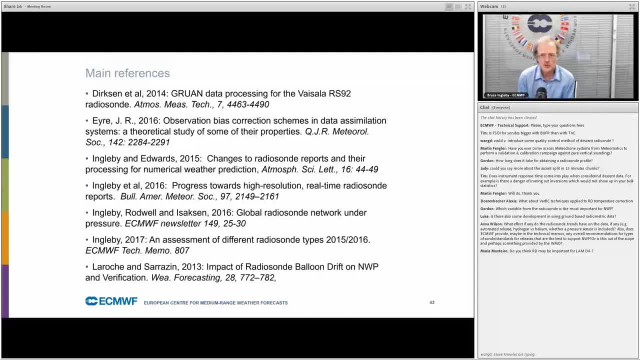 one question from Alexis. It's gone off the top of my screen. Okay, very active. Yes, Let's see if we can. I suppose yes, So Alexis. Okay, Alexis has asked what about VAR-BC techniques applied to radius on. 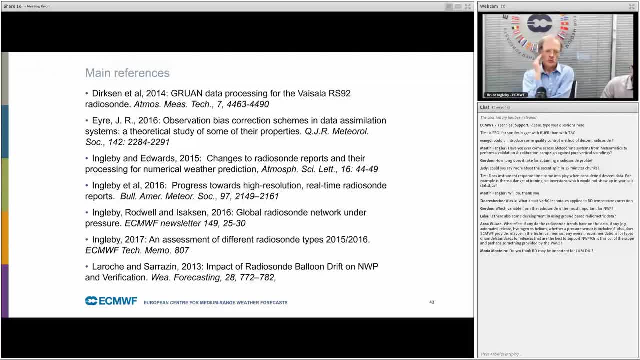 temperature correction. We don't want to use VAR-BC directly for radius ons because that would weaken its role as anchor observations and in general terms I would prefer to reduce the biotic correction, Certainly for modern radius, on types Which variable from radius ons. 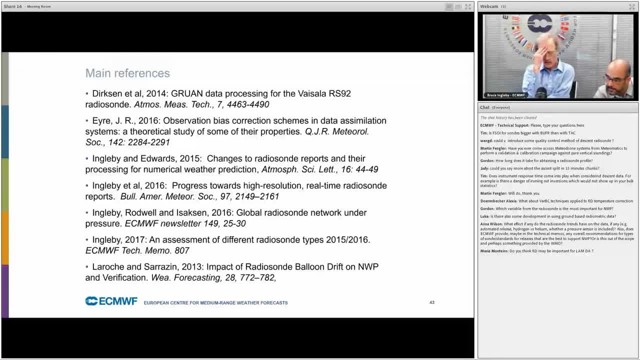 is the most important for NWP, That's. I haven't got a single answer for that and To some extent it varies with latitude In the tropics. we could certainly do with more wind profiles, And we don't see wind profiles from satellites. 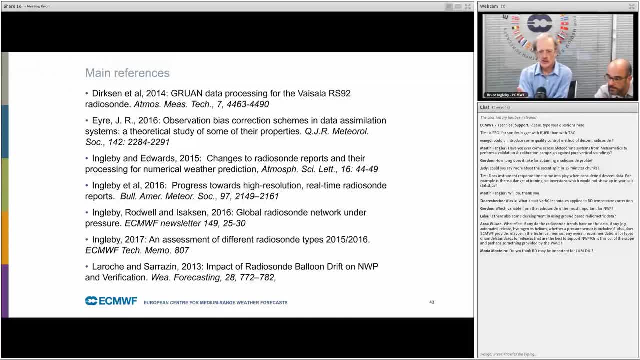 So wind is an important variable for NWP, Temperature is two And humidity actual correctness, of course. OK, I mentioned that quickly. We don't use ground-based radiometric data at the moment. It's not, as far as I know, sent on the GTS. 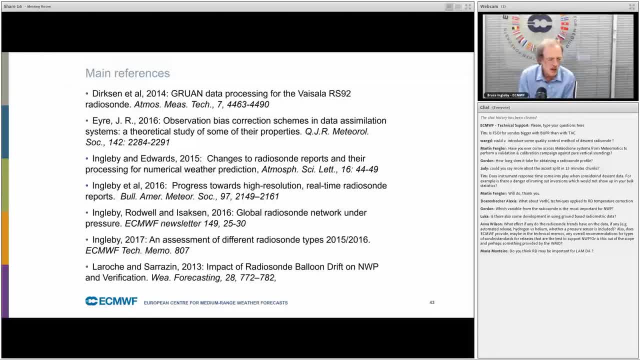 And there aren't many stations providing it. OK, these questions about radius, on trends, Automated data, Automated launch. So the ECMWF? ECMWF doesn't state so much of grief, It doesn't say what it says, It doesn't say how it is. 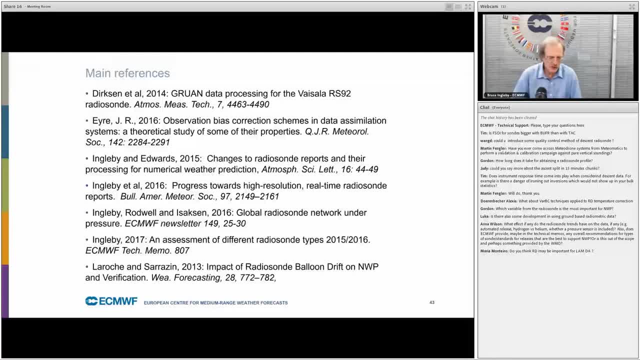 directly provide recommendations for types of radiosondes. I mean you can look at my technical memo and you will see there are a number of good radiosonde types and a number of slightly less good radiosonde types and there are WMO radiosonde into comparisons every so often. There will be another in about two. 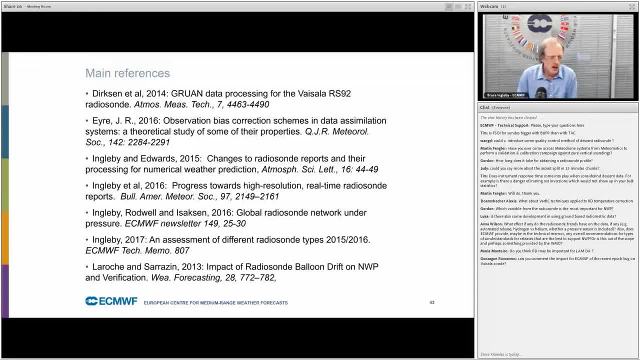 years time. It's certainly not ECMWF's role to directly tell users what radiosonde they should be using. Do I think radiosondes are important for limited areas? They are to some extent, obviously- and things like getting the boundary layer height correct- that they should be very useful. for that There's a 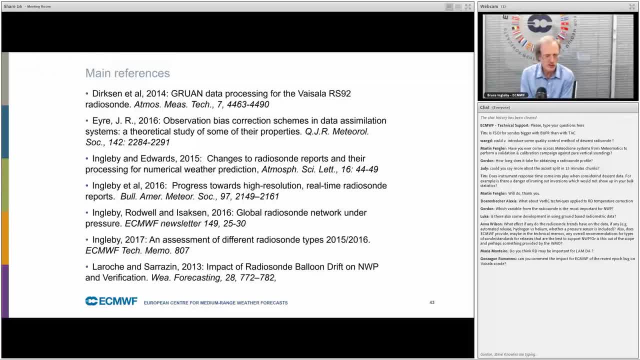 question about the recent GPS epoch rollover which affected a number of Vysala radiosondes, 20 to 30 worldwide. The number of radiosondes was not large and most of them came back relatively soon, So I don't think it was that large. It was unfortunate, of course, and we did see. 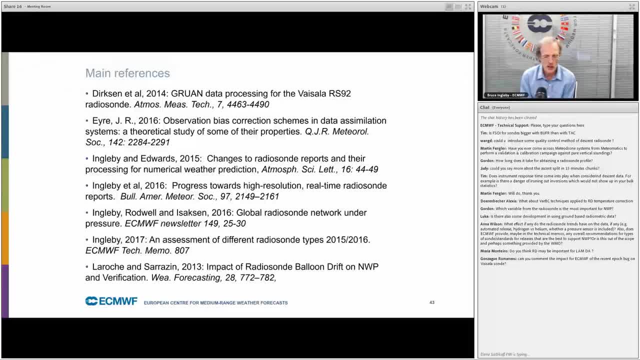 some loss of drifting void apes as well. Thank you, Thank you, Thanks a lot again. fairly small. There are few observations in polar regions. Is it necessary to get radius on data there for improving NWP scale? It would help. 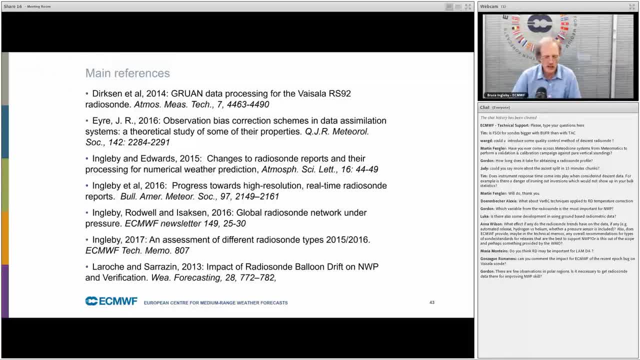 As you may know, there's been a year of polar prediction going on recently, with extra releases in the Arctic area and it's now in the Antarctic. One of the answers is: it depends how many customers you have. adow pit, I guess one of the answers: it depends how many customers you have. How many they have in the Arctic, as to how much effort you want to spend there And the year of polar prediction. the APLICATE project will be doing tests with and without Arctic radiosondes to try to address this sort of question. I don't think I can say anything more on that. Where are we GPS? 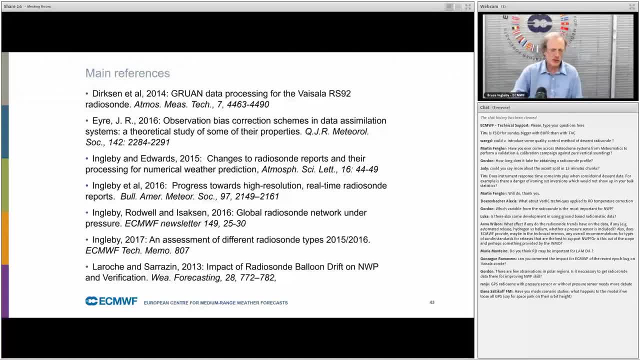 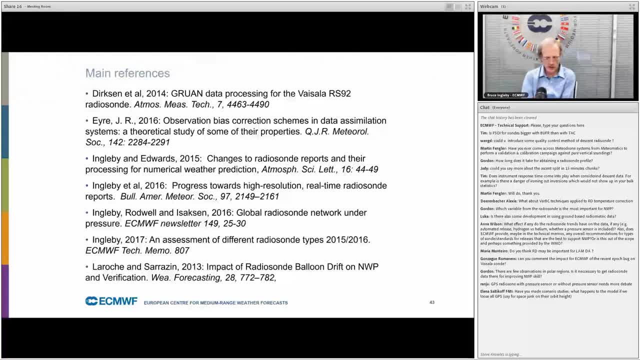